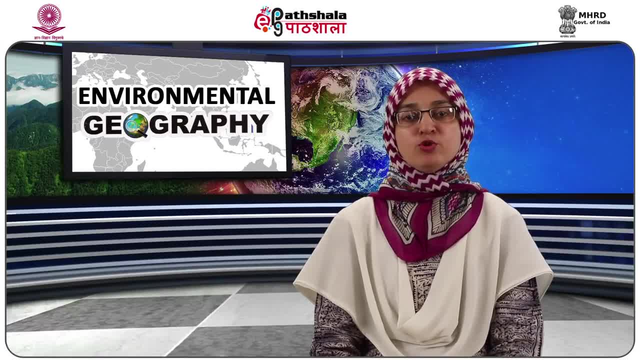 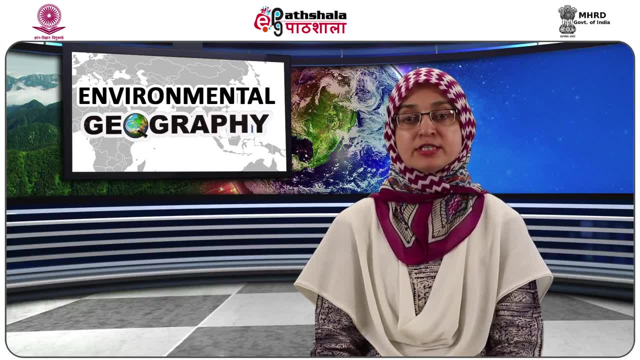 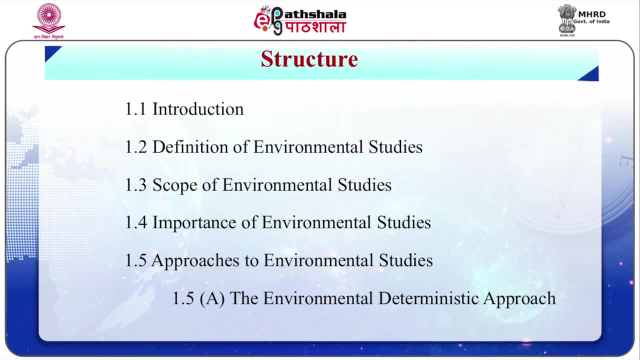 Geography. The objectives of this module are: at the end of this module, the students should be able to define what is environmental study Number 2,. explain the nature and scope of environmental study. Number 3, have clear understanding about the importance of environmental 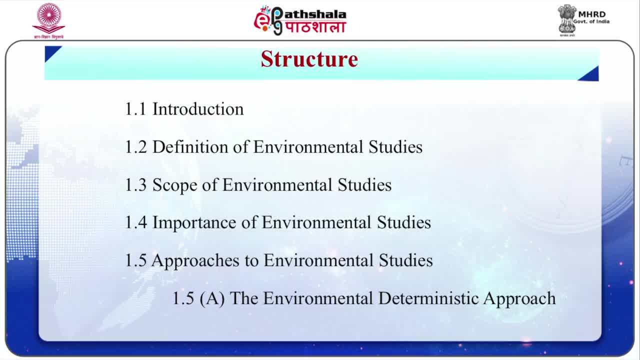 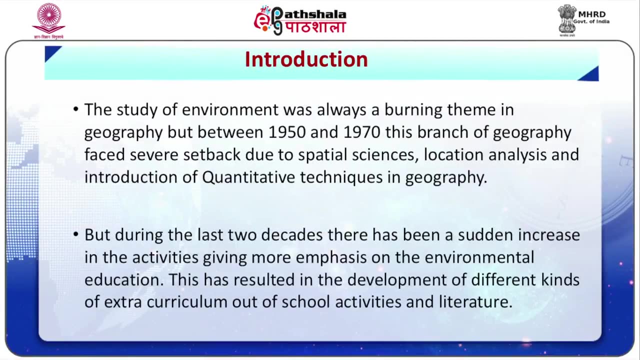 studies. Number 4, explain different approaches to understand environmental studies. Now introduction: the study of environment was always a burning theme in geography, but during the period between 1950 and 1970, this branch of geography faced sea-following challenges. 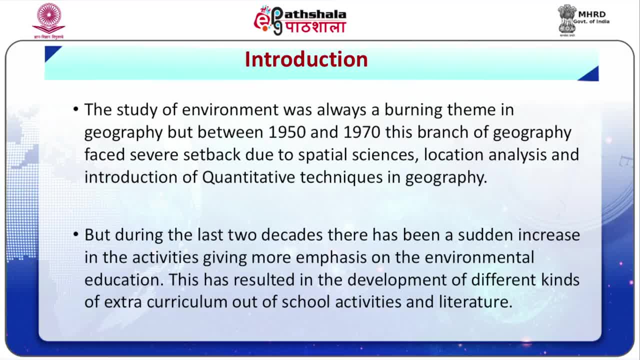 There was a severe setback due to spatial sciences and location analysis, and also because of the introduction of quantitative revolution in geography, which promoted the use of statistical techniques in geography, according to Singh, 2006.. But during the last two decades, there has been a sudden increase in the activities, giving more emphasis on the environmental 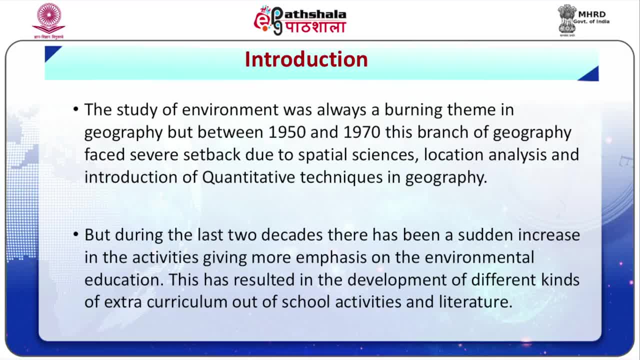 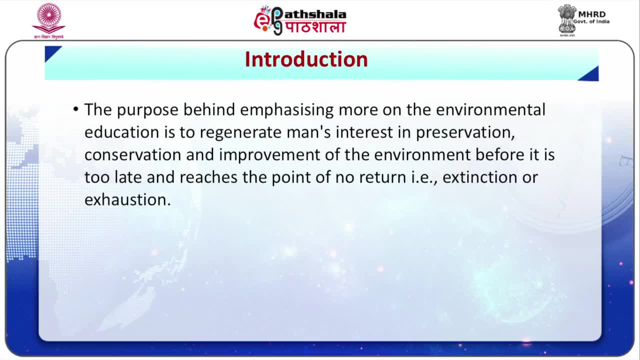 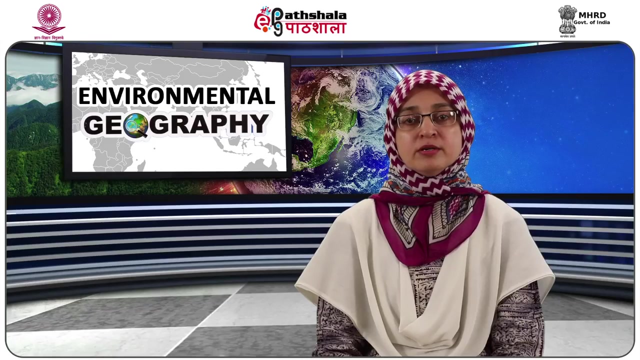 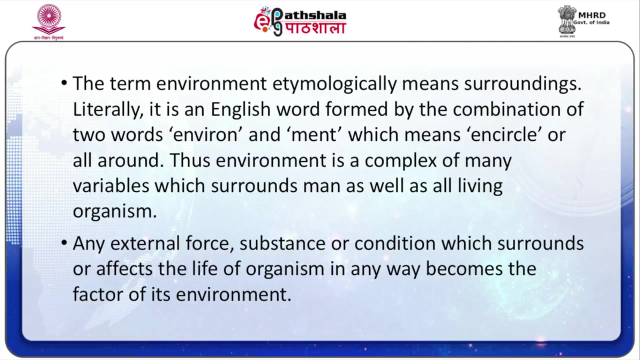 education. The word environment etymologically means surroundings. Literally it is an English word. The word environment is derived from French word environ, which means surrounding, formed by the combination of two words environ and ment, which means encircle or all around. Thus, environment is a complex of many variables which surrounds man as well as all living organisms. 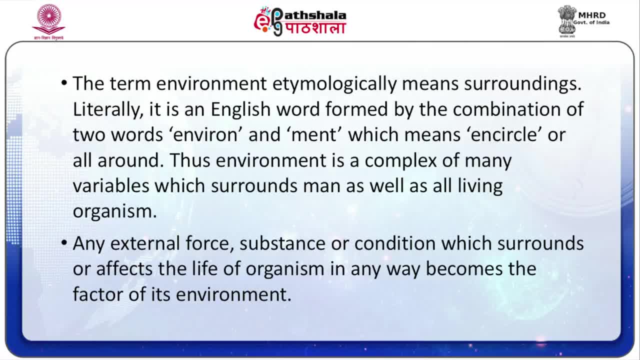 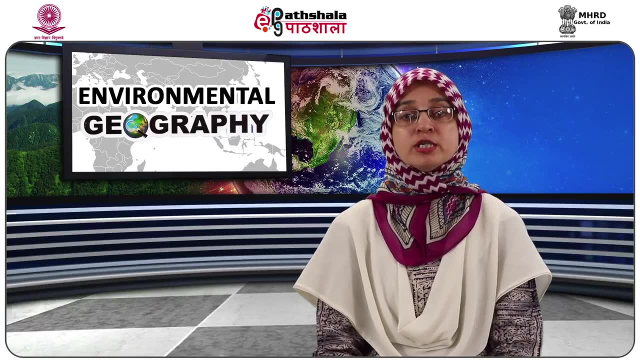 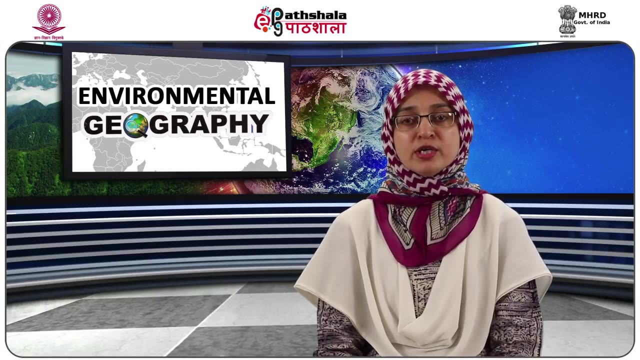 Any external force, substance or condition which surrounds or affects the life of organism in any way becomes the factor of its environment. The place where an organism lives is called habitat. It is also known as milieu, which means total set of surroundings, according to Saxena 2004.. 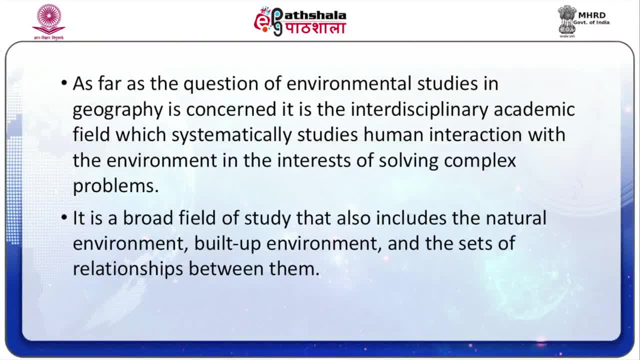 Number 4, have clear understanding about the importance of environmental studies. As the question of environmental studies in geography is concerned, it is the interdisciplinary academic field which systematically studies human interaction with the environment in the interest of solving complex problems. It is a broad field of study that also includes 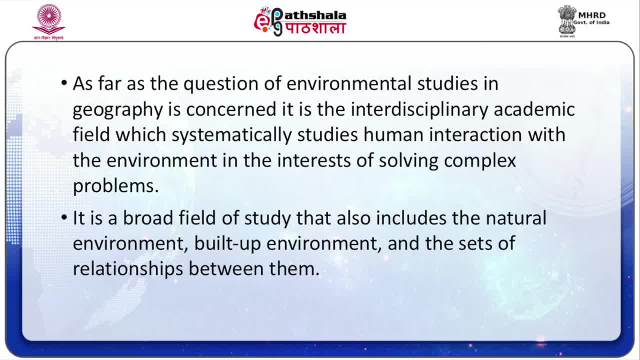 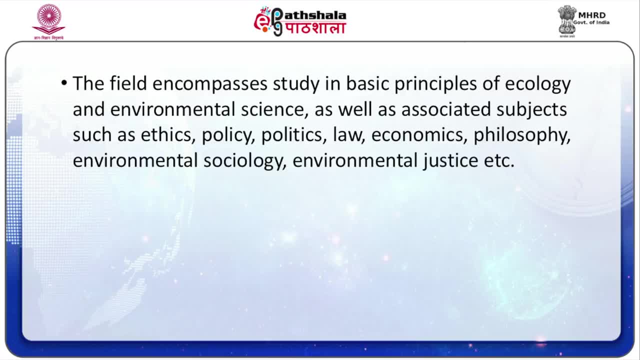 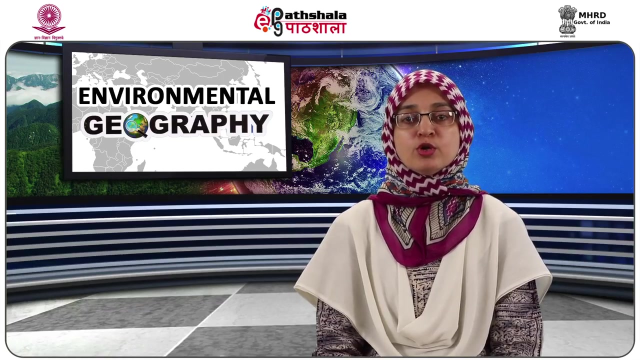 the natural environment, built up environment and the sets of relationships between them. The field encompasses study in basic principles of ecology and environmental science, as well as associated subjects such as ethics, policy, politics, law, economics, philosophy, environmental sociology and environmental justice planning, pollution control and natural resource management. 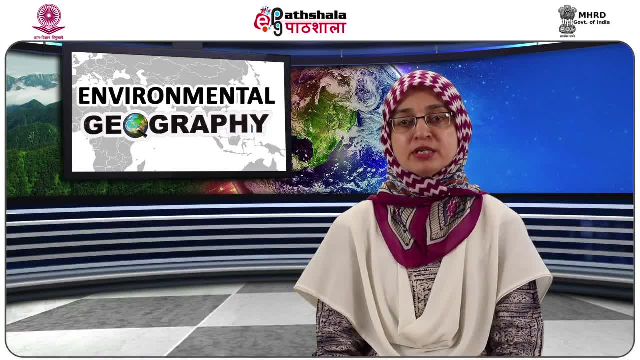 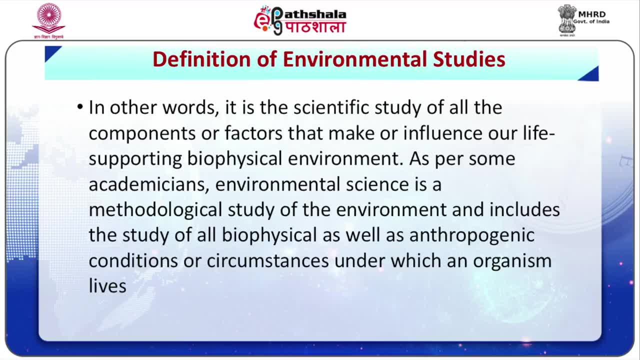 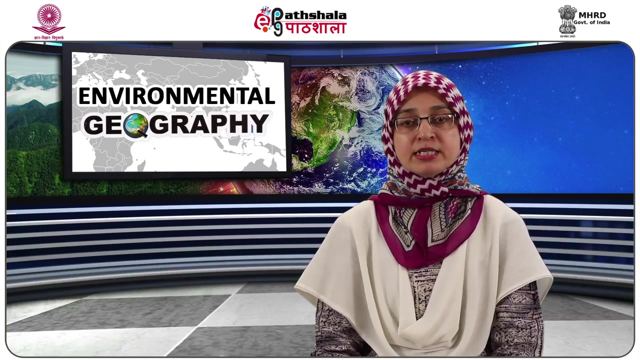 Number 5, definition of environmental studies. 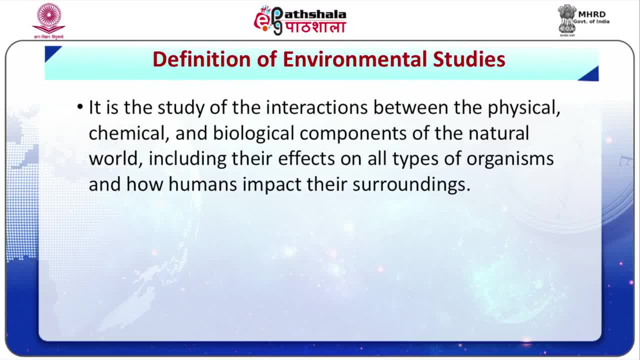 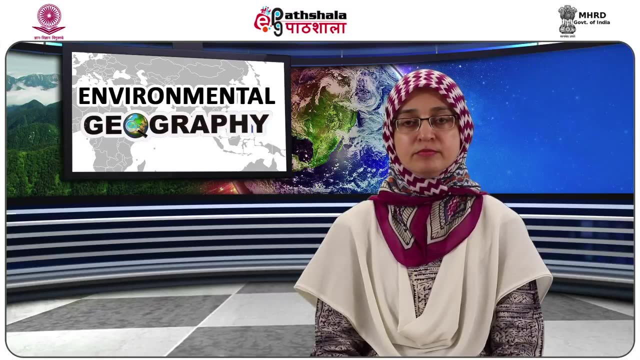 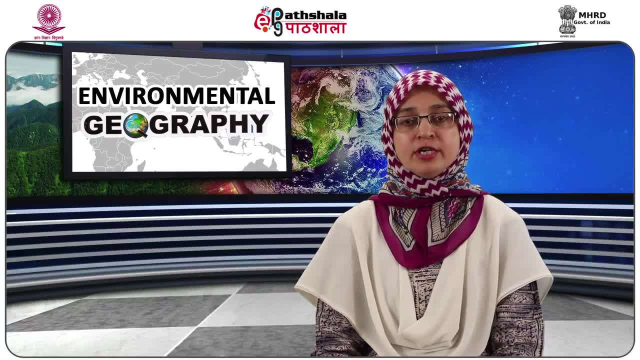 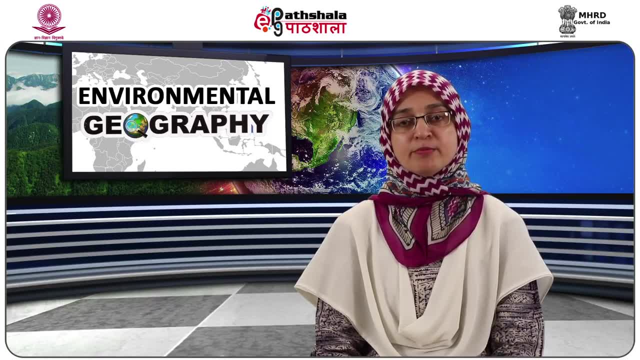 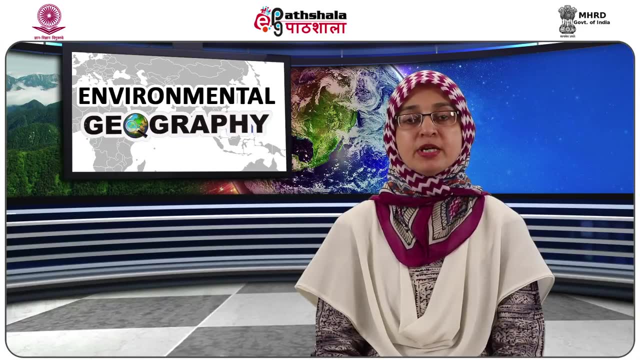 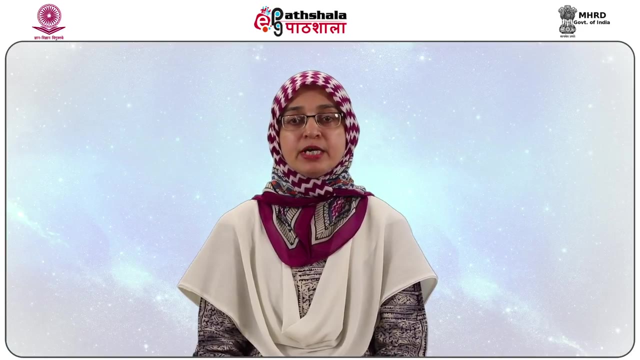 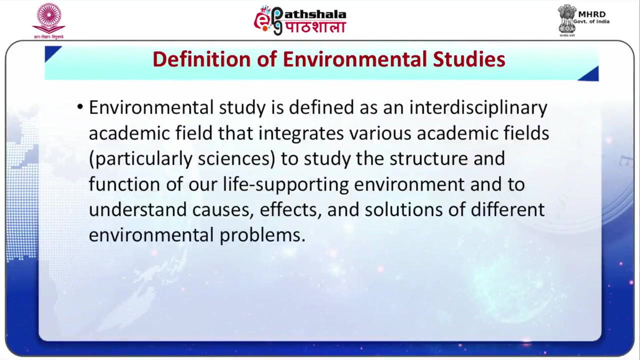 phenomena in the environment, according to Singh 2006.. Environmental study is defined as an interdisciplinary academic field that integrates various academic fields, particularly sciences, to study the structure and function of our life, supporting 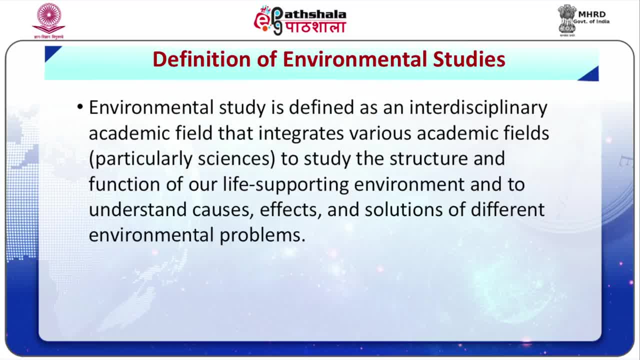 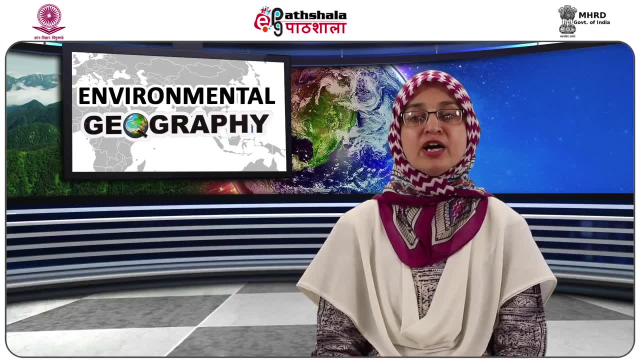 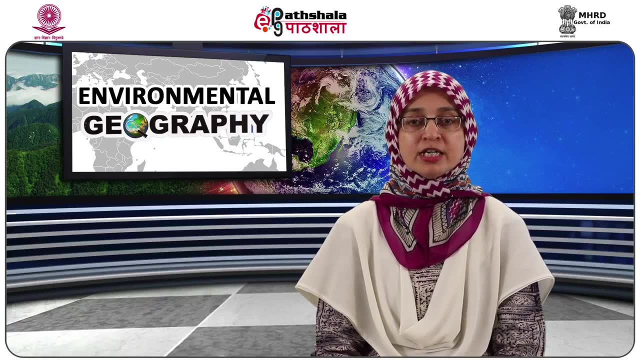 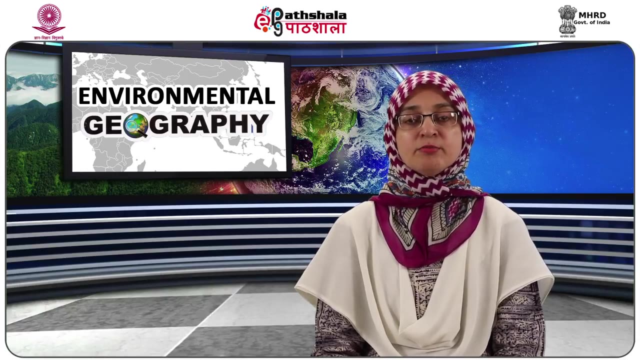 environment and to understand causes, effects and solutions of different environmental problems. Now the scope of environmental studies. The scope of environmental studies is vast and wide. Sky is its limit and ocean is its depth. What is not covered in environmental studies shall take years and years yet to think as. 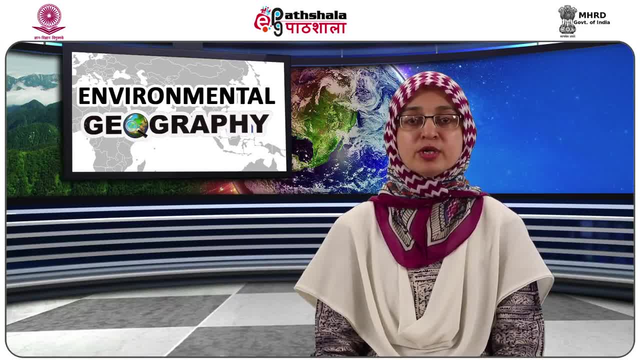 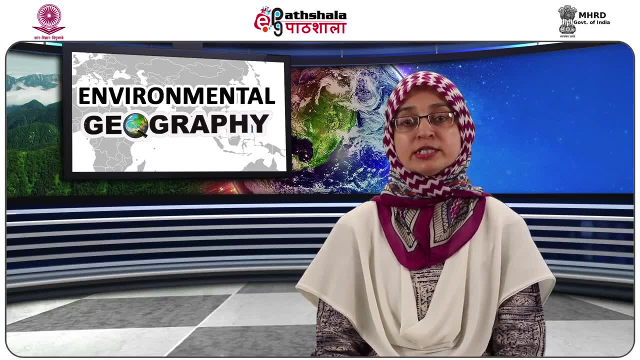 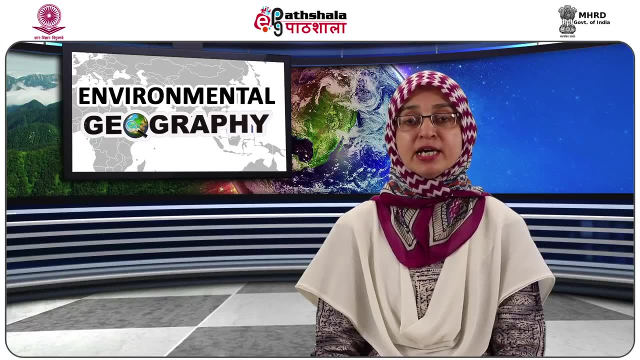 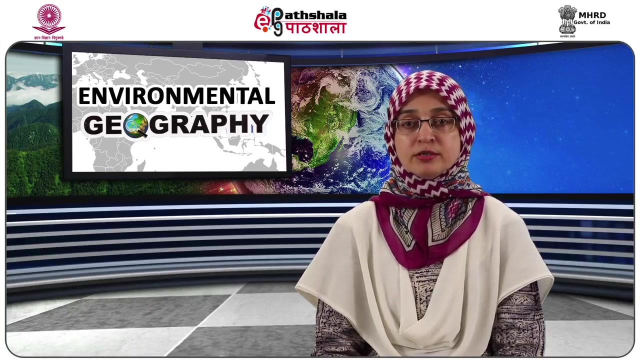 how to cover. Studies reveal that during the past few decades, there has been fundamental change in the attitude of man towards environment. There was a time when environment meant only sanitation and health. Environmental studies teach us about deforestation and forest conservation. Environmental studies teach us about diversified ecologies. 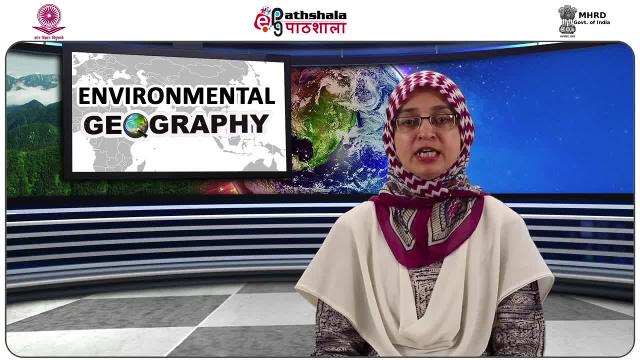 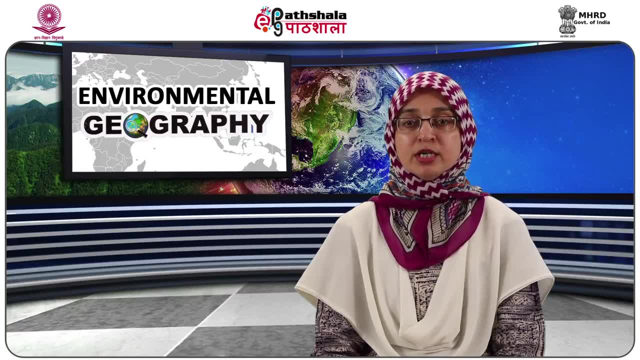 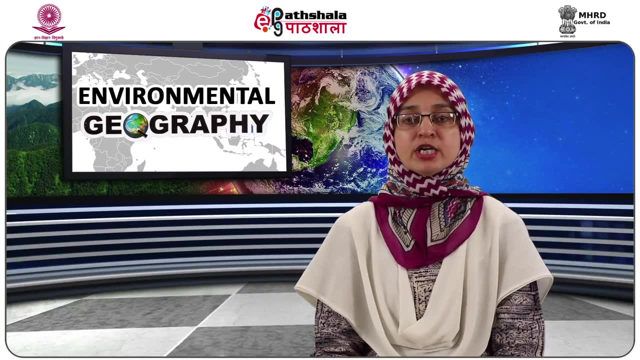 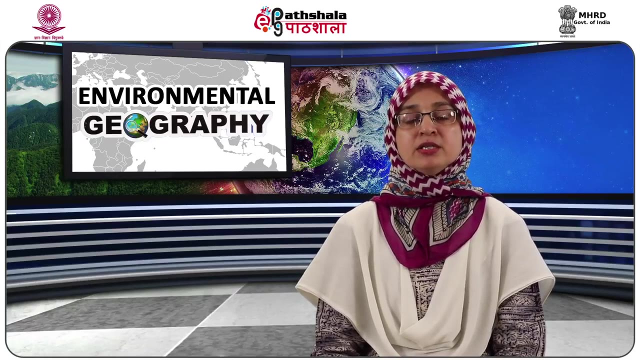 The scope of the environmental study is diverse, dealing with the area such as the geo ecosystem, or simply ecosystem, as a study unit, the functioning of ecosystem, including circulation of energy and matter and ecosystem productivity, temporal changes in ecosystem, evolution of plants and animals and ecological succession, spatial ecological changes, distribution and dispersion. 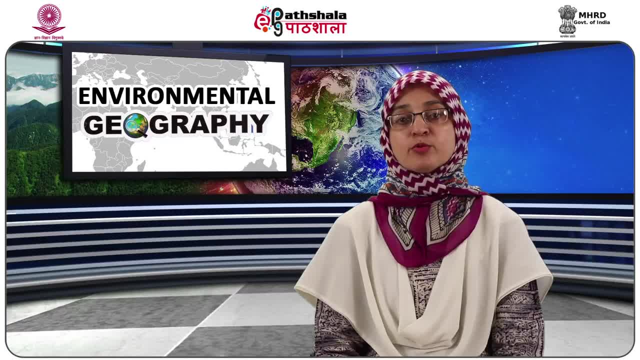 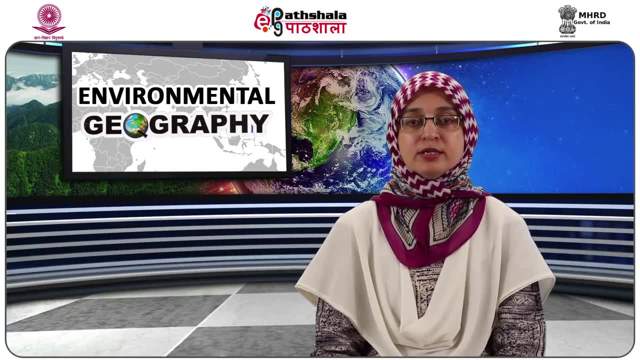 of plants and animals, global environmental problems. The scope of the environmental study is vast and wide. What is not covered in environmental studies shall take years and years yet to think as how to cover. beiš has taxes, environmental hazards and disasters, man and environmental processes. 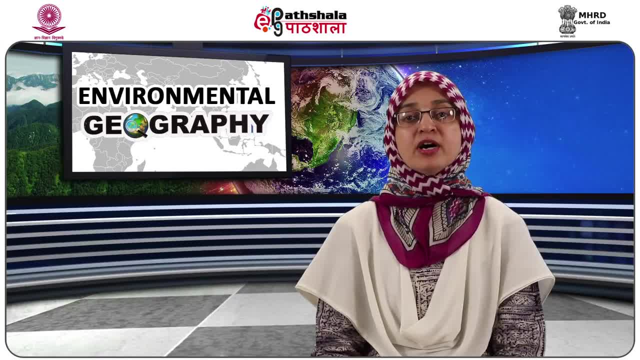 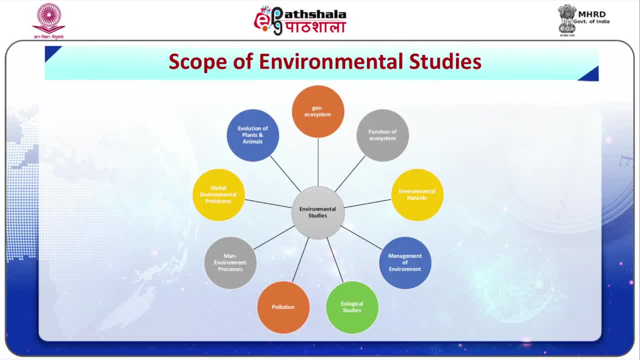 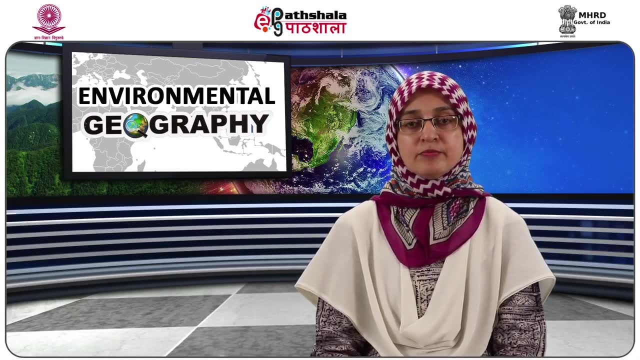 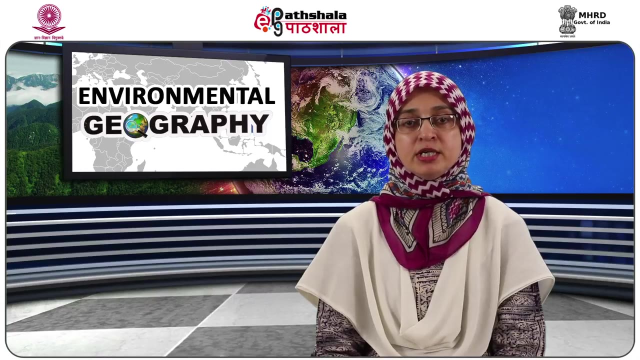 environmental degradation and pollution and environmental management. Slide 10, Figure 1, shows the scope of Environmental studies. Now the importance of Environmental studies. Vari Dahabunoji, Various combinations of words, such as environmental, Environmental education, that is EA, environmental study, that is ES, and environmental approach. 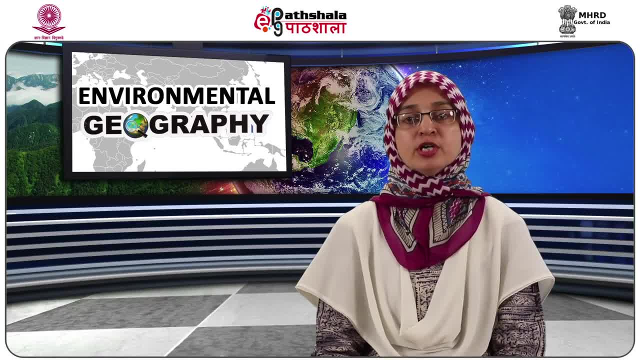 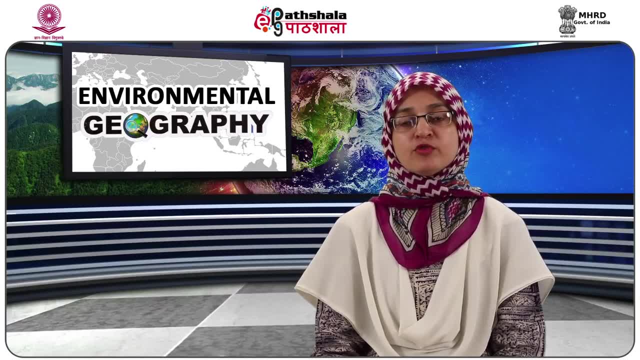 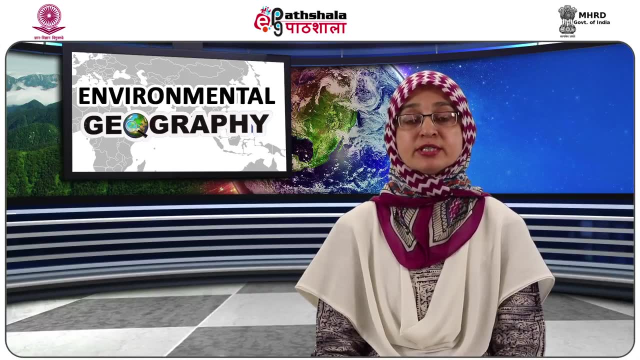 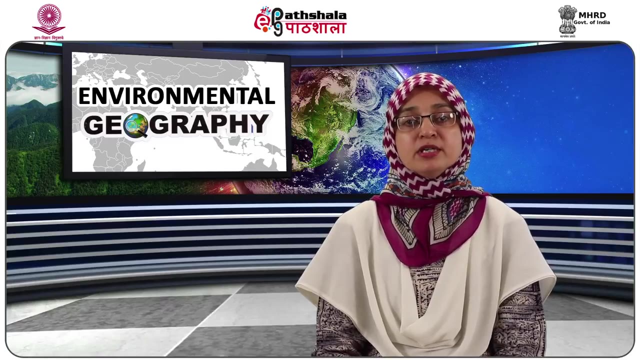 that is, EA, are being used in the literature in the context of environment and education, Although according to semantics of the words, EE, ES and EA have different meanings in the strict sense of the terms, but one finds that these are being used many a time synonymously. 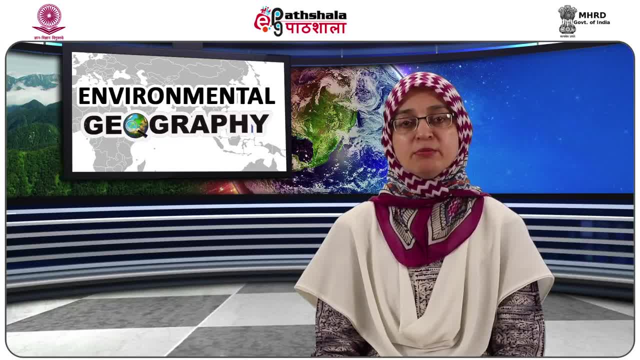 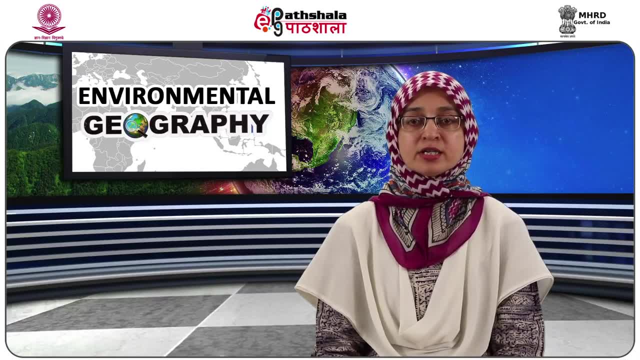 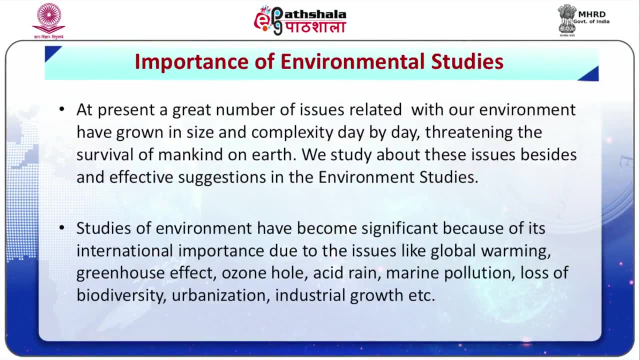 and interchangeably. The environmental studies enlighten us about the importance of protection and conservation of our indiscriminate release of pollution into the environment. At present, a great number of environmental issues have grown in size and complexity Day by day, threatening the survival of mankind on earth. 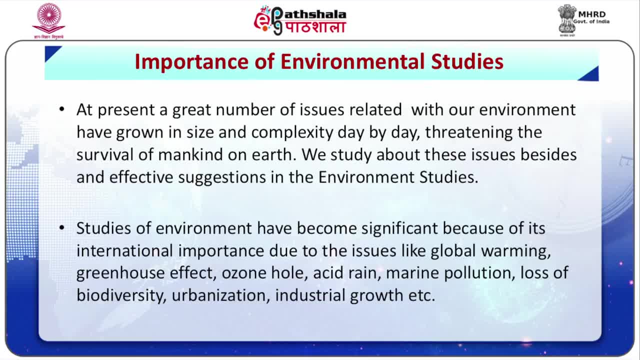 We study about these issues besides an effective suggestions in the environmental studies. Environmental studies have become significant because of it is international importance due to the environmental issues like global warming, green house effect, ozone hole, acid rain, marine pollution and heat auf. 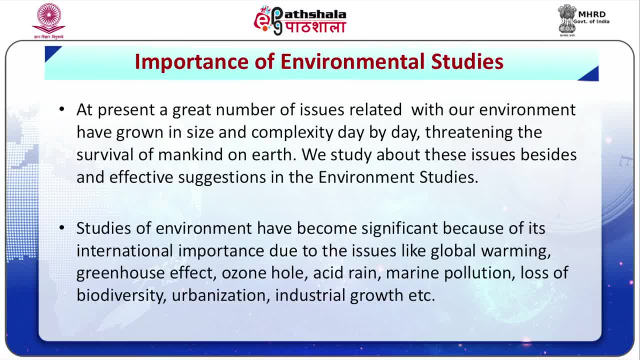 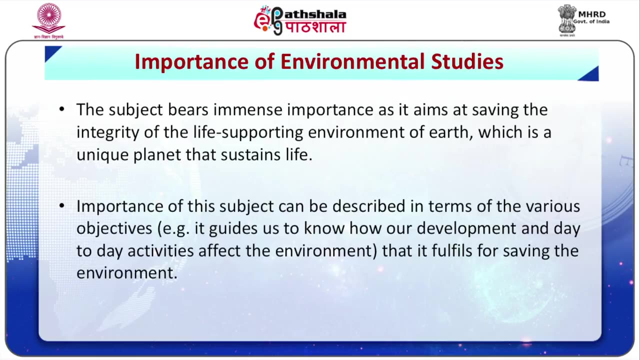 and loss of biodiversity. Environmental studies are also necessary because of the problems arising out due to development and its phenomenon, like urbanization, industrial growth, construction of expressways, subways and highways. The subject bears immense importance as it aims at saving the integrity of the life, supporting 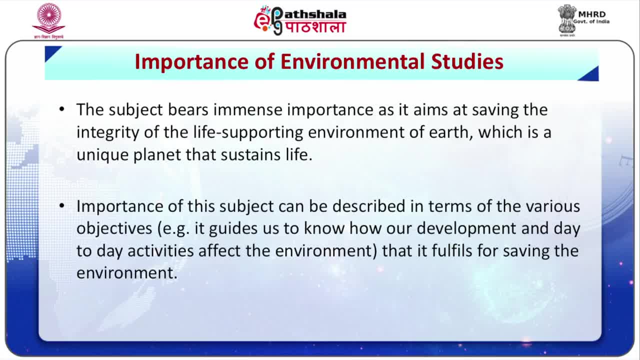 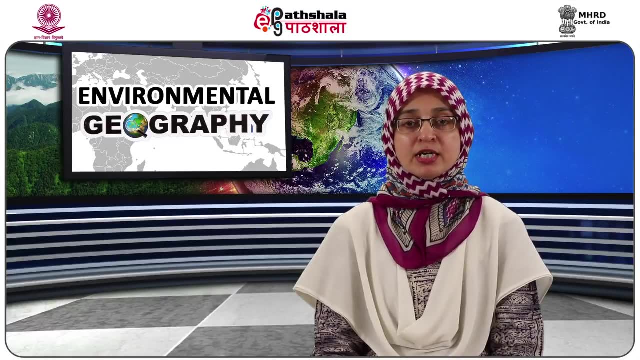 environment of earth, which is a unique planet that sustains life. Importance of this subject can be described in terms of the various objectives that it fulfils for saving the environment. Some of these objectives are that it guides us to know how our development and day to 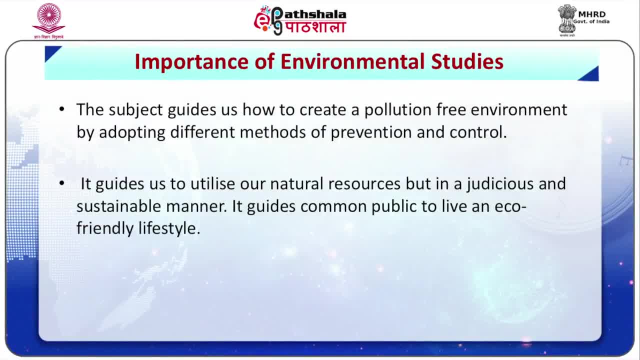 day activities affect the environment. The subject guides us how to create a pollution climate. The subject guides us how to create a pollution-free environment by adopting different methods of prevention and control, and it also guides us to create pollution-free environment. It guides us to utilize our natural resources, but in a judicious and sustainable manner. 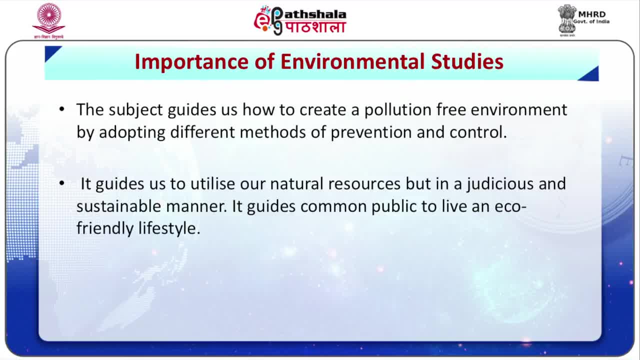 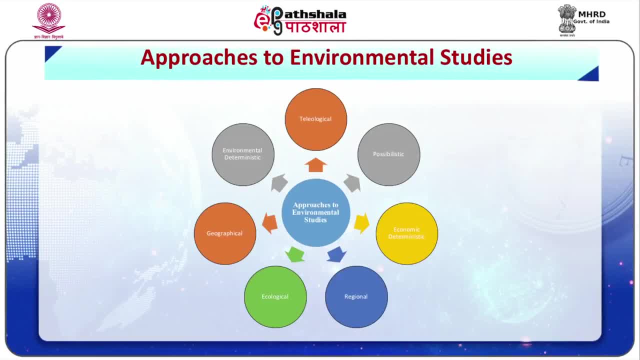 It guides common public to live an eco-friendly lifestyle. Now approaches to environmental studies. An approach is a way of getting closer. The study of relationships between man and environment has always been, in one way or another, a focal theme in environmental study. but the facets of man-environment relationship, 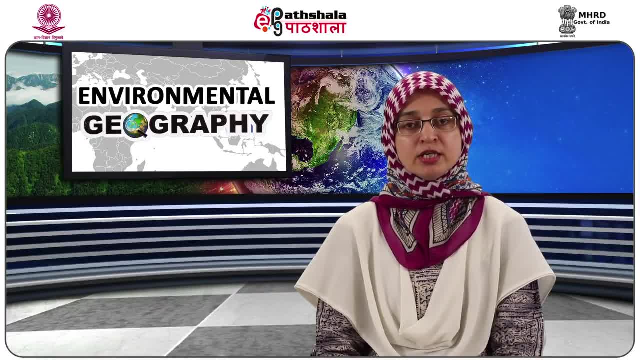 changed through time with the development of human society and the dimension of the environment, As the man became social, economic, environmental, mechanic. he discussed species and the environment. Hi Edu AustinærLaughterß an approach zu der Lusten herum: die Gesellschaft. 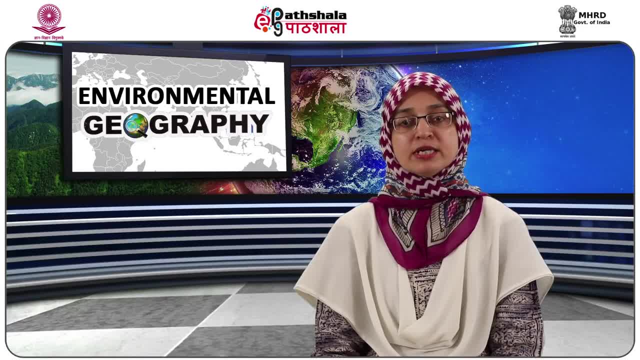 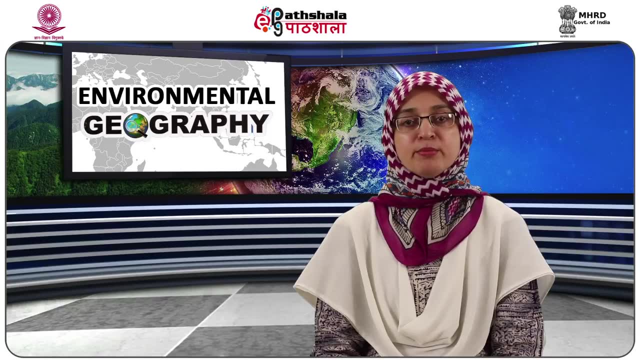 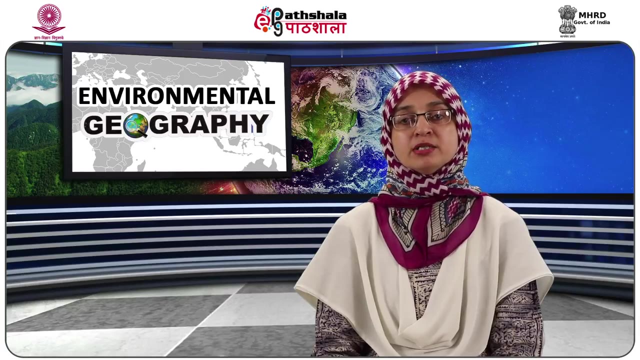 economic and technological. he broadened his environment by creating his own environment through his designs and skills to have provision for better food, shelter, access and comfort. The man-environment relationship thus can be perceived and evaluated in a variety of ways and approaches. 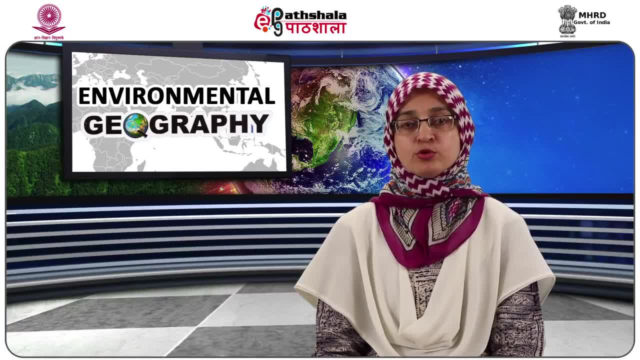 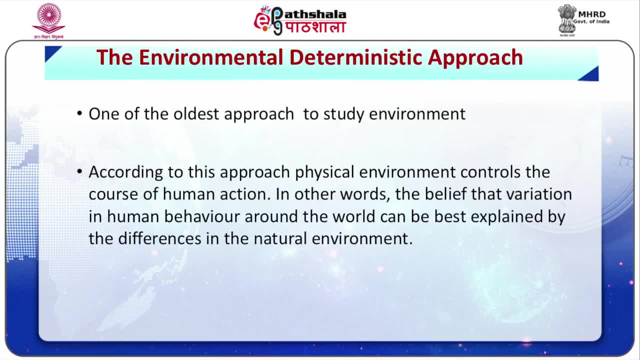 Number 1, the environmental deterministic approach. Deterministic approach is one of the oldest approaches to study environment. According to this approach, physical environment controls the course of human action. In other words, the belief that variation in human behavior around the world can be. 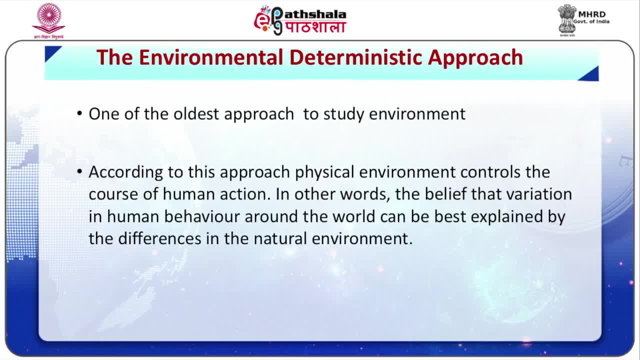 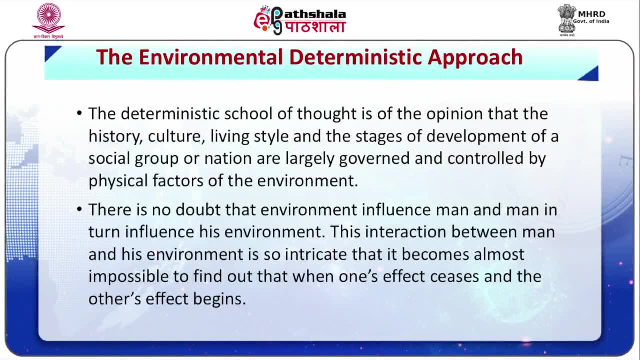 explained by the differences in the natural environment, is the crux of this matter. Number 2, the man-environment relationship. philosophy, The deterministic school of thought, is of the opinion that the history, culture, living style and the stages of development of a social group or nation are largely governed and controlled. 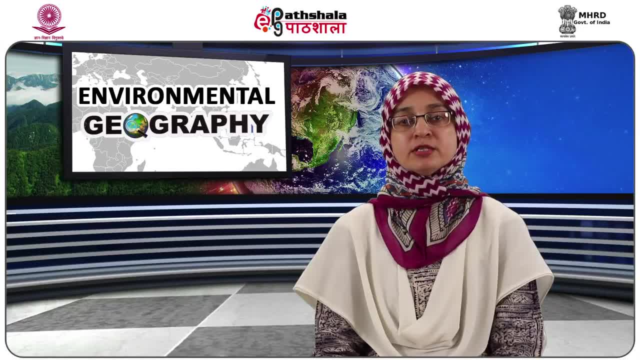 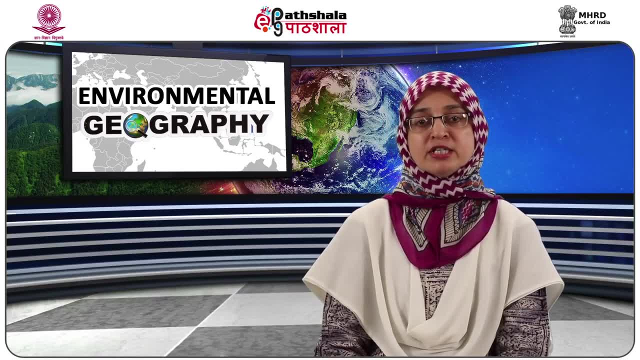 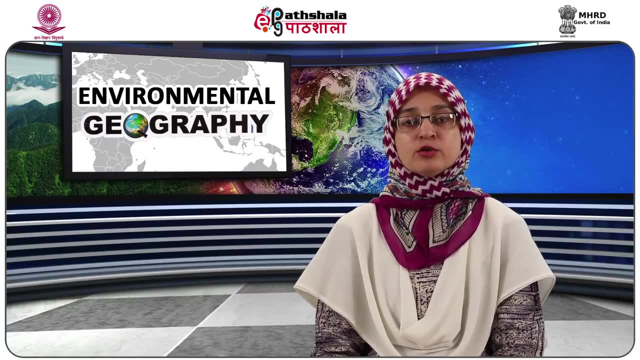 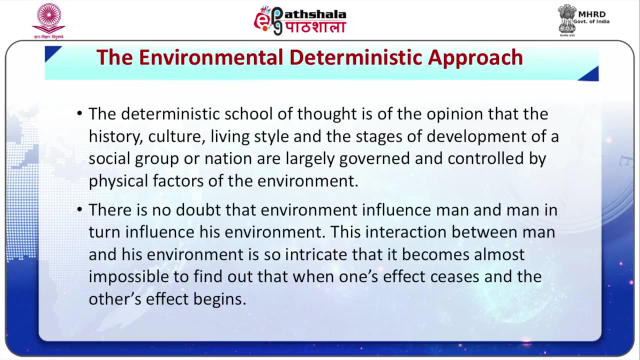 by physical factors of the environment. This philosophy says that aspects of physical geography, particularly climate, influence set of individuals, which in turn defined the behavior and culture of the society that those individuals formed. For example, tropical climates were said to cause laziness, relaxed attitudes and promiscuity. 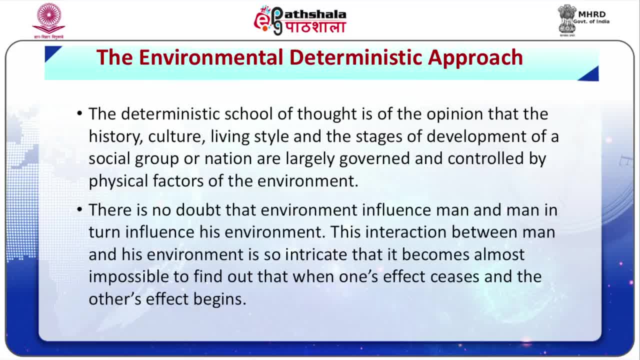 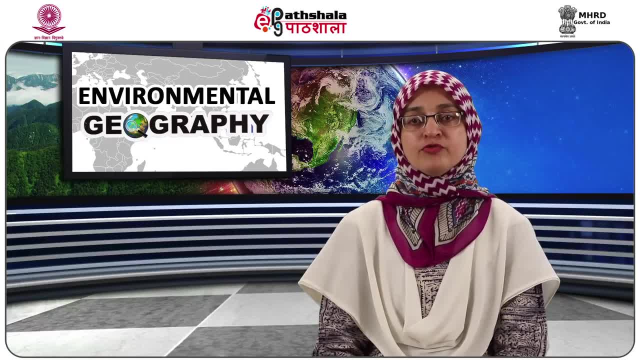 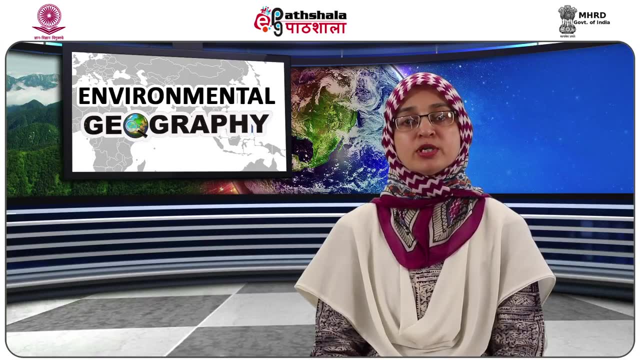 while the frequent variability in the weather of the middle latitudes led to more determined and driven work ethics. This philosophy supports the idea that the highest achievement of civilizations like Egyptians, Mesopotamians, Indus Valley disappeared because of the climatic change. 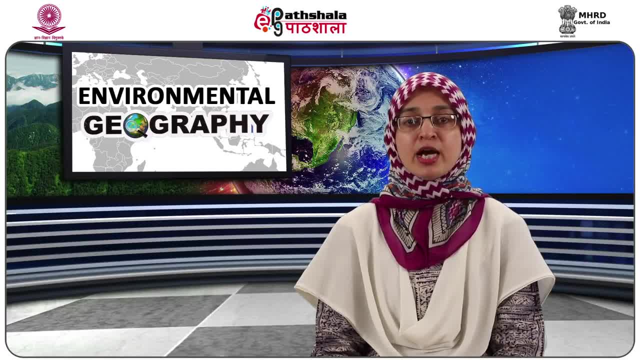 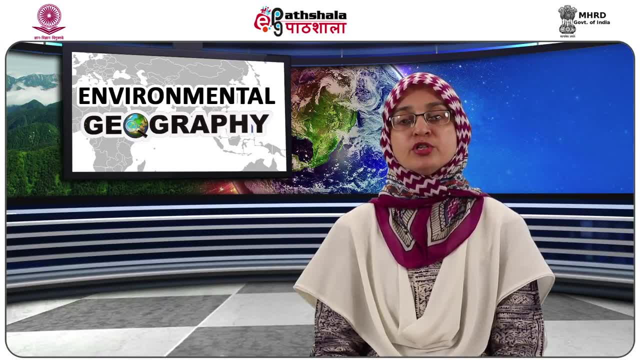 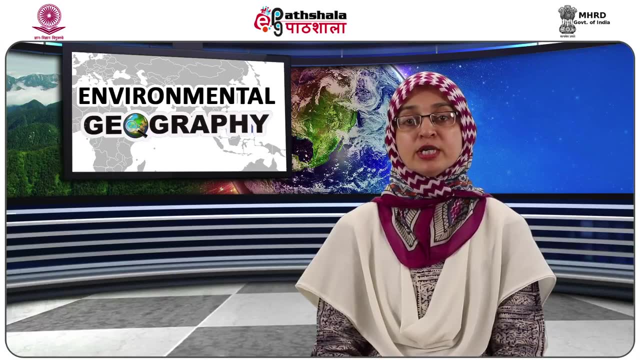 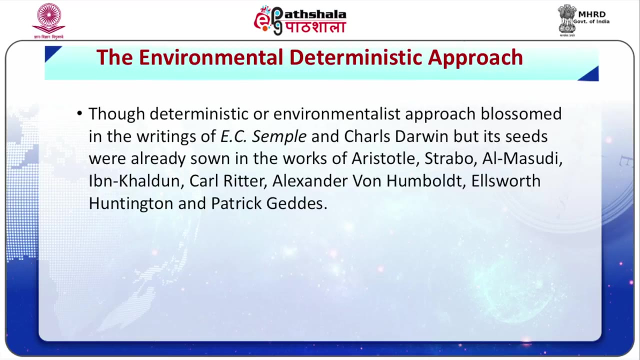 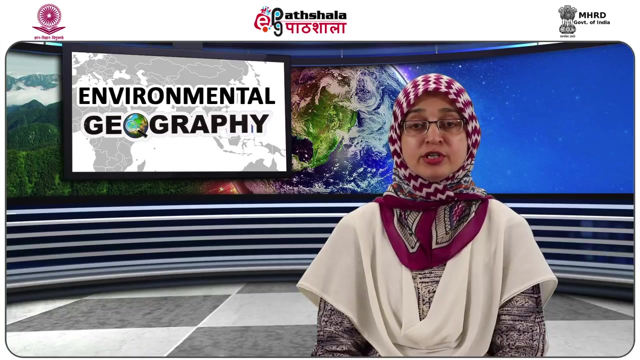 It is also believed that the attack of Central Asian nomads on other civilization is because of change in climate, because it was climate change which resulted into the drying up of their pastures, which forced them more to live in the desert. The 19th century. 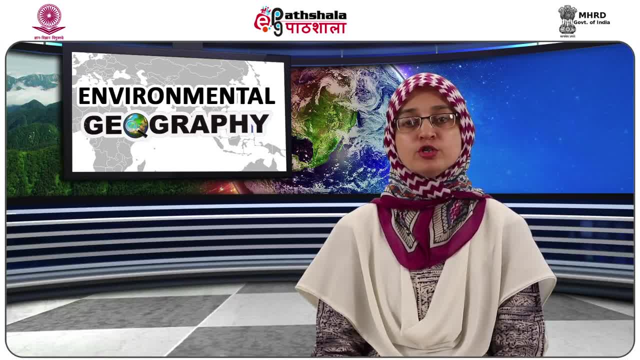 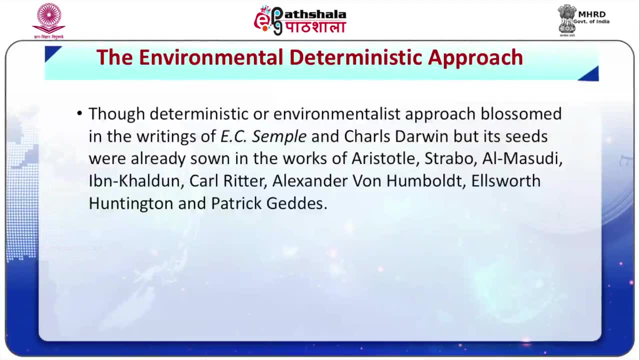 In fact, the publication of the Origin of Species of Charles Darwin in 1859, the first publication of the Origin of Species of Charles Darwin in 1859, laid the foundational stone of the concept of environmental influences on man and other organisms, and even before. 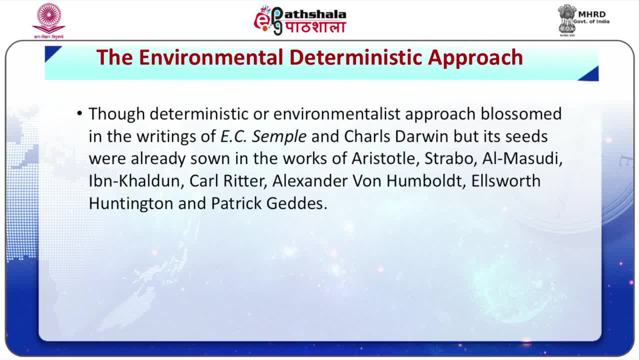 that the seeds of determinism was found in the works of Aristotle, Strabo, Al-Masudi, Ibn Khaldun, Carl Ritter, Alexander I Humboldt, Ellsworth, Huntington and Patrick Geats. There is no doubt that environment influenced man and man in turn influenced the climatization. 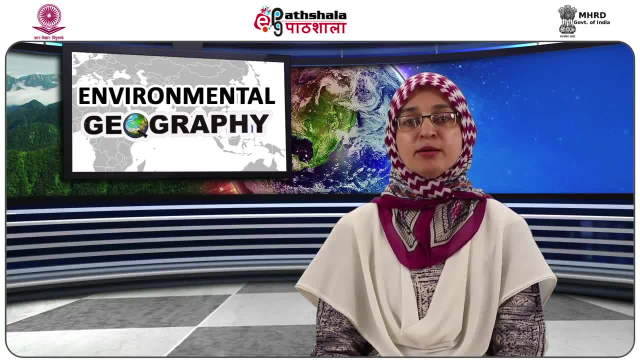 The establishment of the first scientific organization in the world, which was the early civilization, was the foundation of the idea of environmental influences. The first scientific organization was the early civilization. the first scientific organization, which was the early civilization, in turn influence his environment. 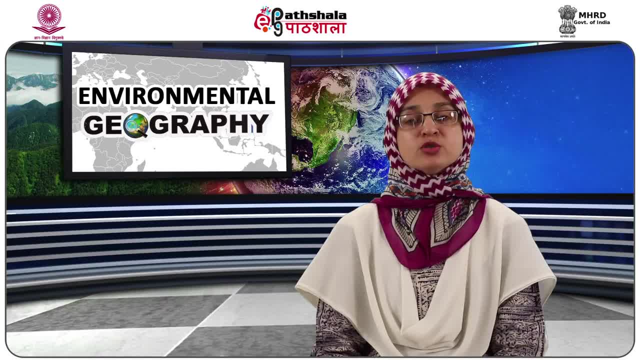 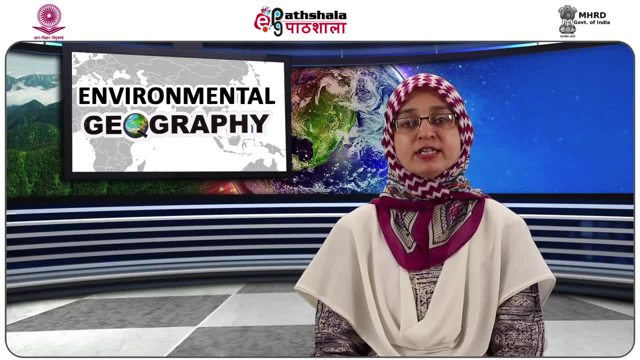 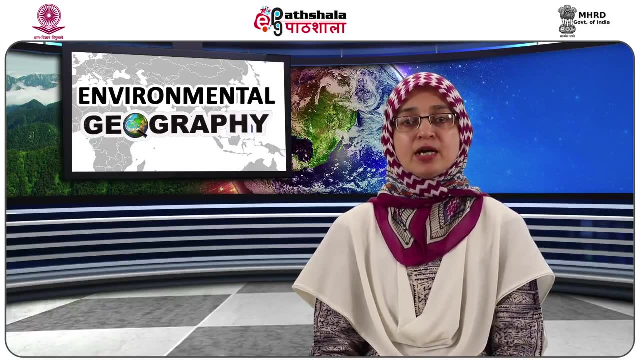 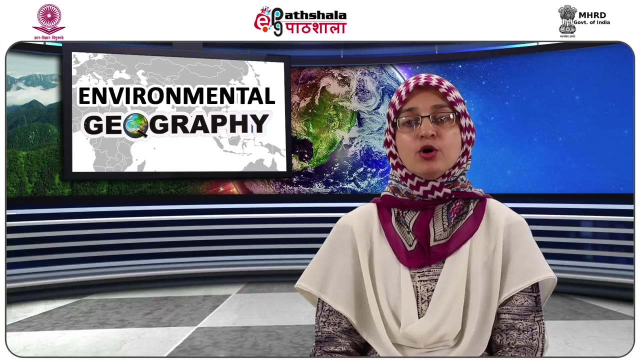 This interaction between man and his environment is so intricate that it becomes almost impossible to find out that, when one's effect ceases and the other's effect begins, Many landscapes that appear natural to us are in truth the work of man. wheat barley. 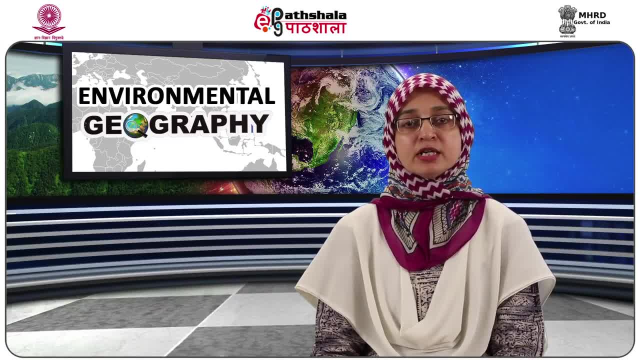 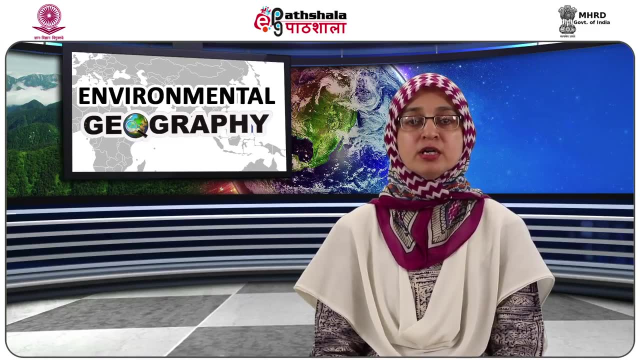 olive and wine which dominate the Mediterranean countries are entirely the products of human effort. Apple and almond orchards of Indian states, for example Kashmir, Himachal Pradesh and Kumamon division of Uttarakhand, are the creations of man. Many geographers in the United States, Britain, Canada and other countries drew attention. 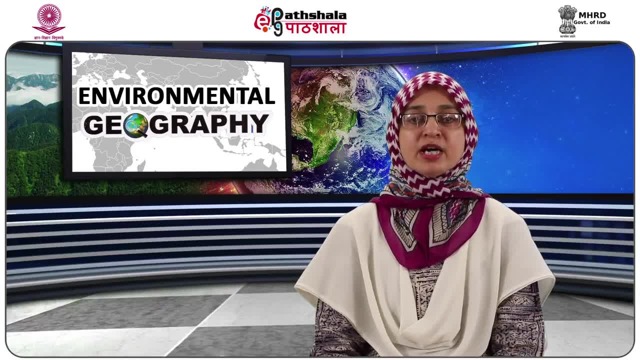 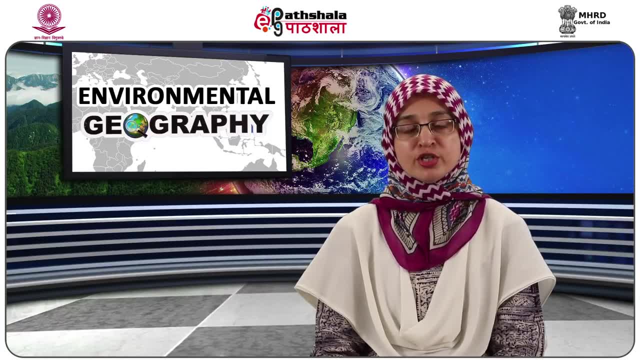 to the one-sided approach. Today, the word man is used terminally in the film by his local writer, AC Blackburn. In fact, it is his own interpretation of a word that is adopted by the environmentalists in their interpretation of historical reality to their exaggeration of nature's active. 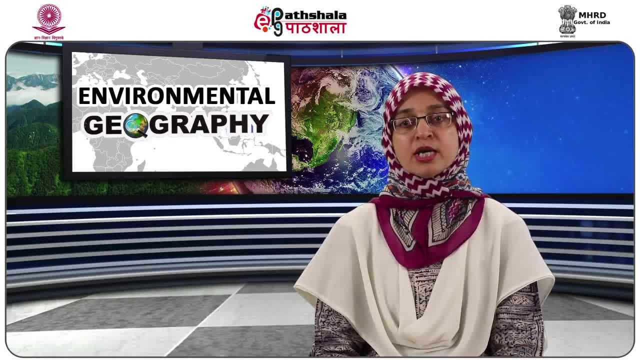 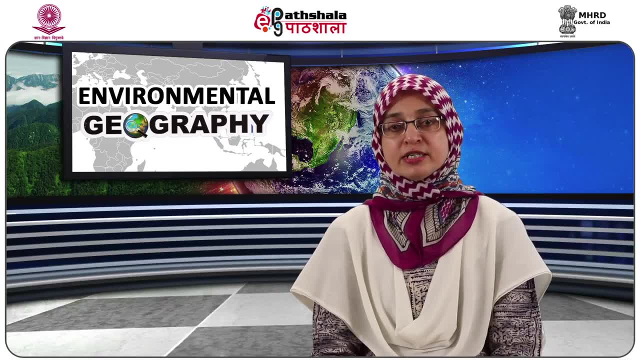 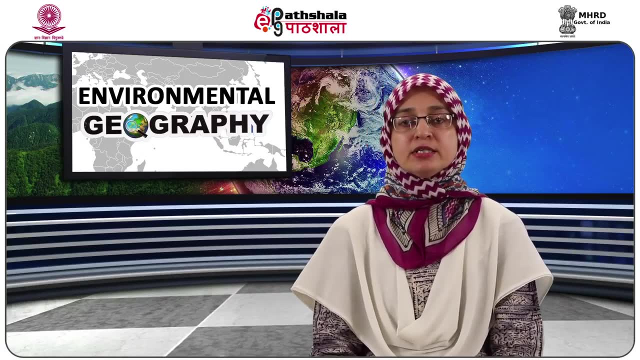 role and to the fact that they only knowledge man as capable of passive attempts at adaptation. Actions of man reveal many facts. Cate criticizes the fanatic approach of environmental deterministic. He, for example, states that environment taken by it is a meaningless phase without man. 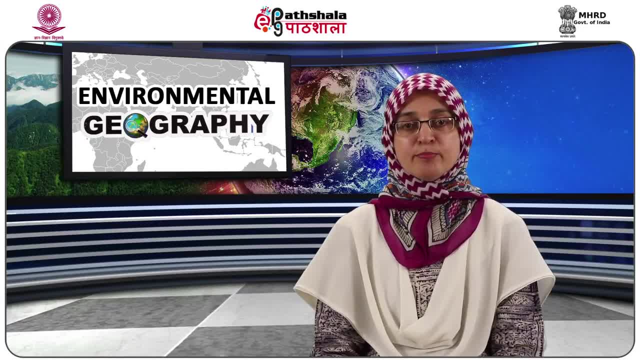 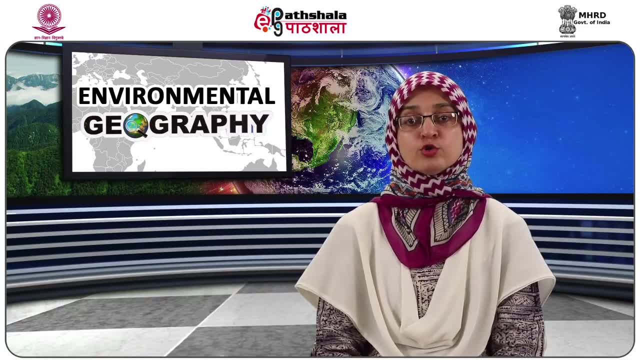 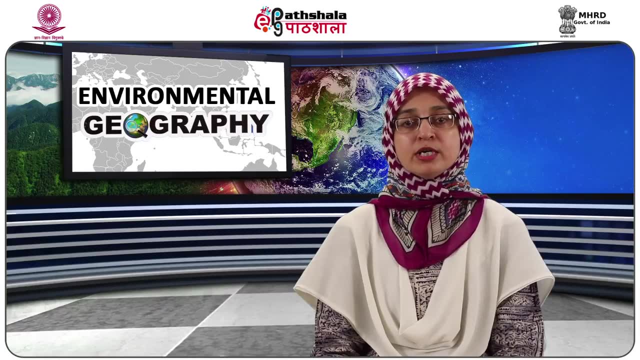 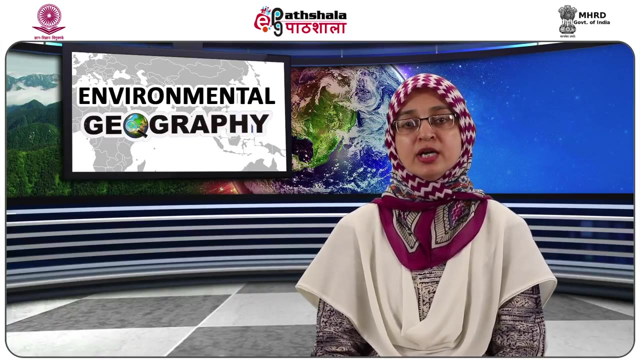 environment does not exist. Equally important is his indication of the need to consider the psycho-physiological influence of the geographical environment via the social structure. In the final analysis, Speyth concluded that geographical environment is only one of the factors of territorial differentiation and it acts through society, cultural tradition. 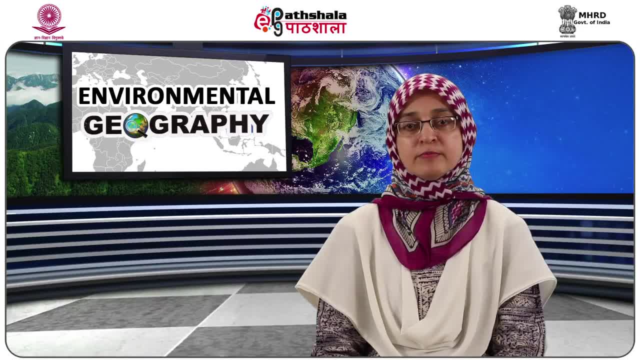 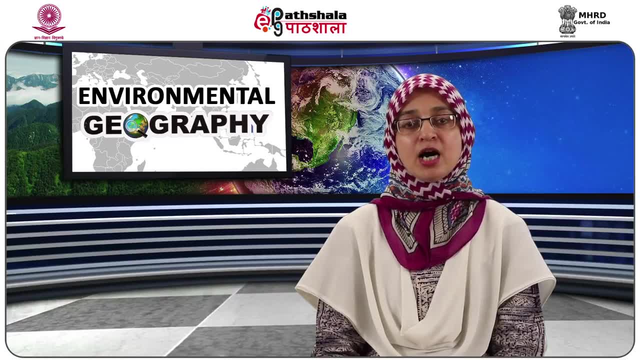 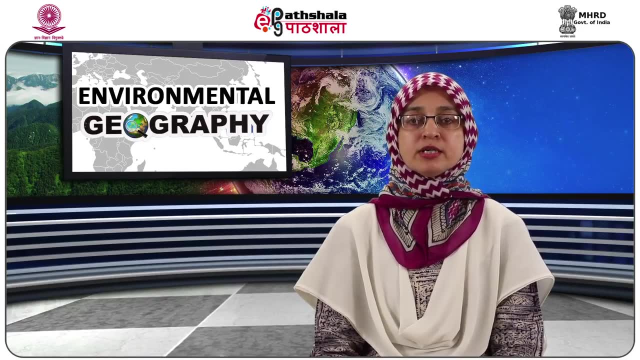 has a certain autonomous influence. The environmentalist movement started in the 1960s has, however, shown quite distinctly that there is an overall awareness- Urgently we should agree- that there is a mouth and a negative thinking limit to certain kinds of human economic activity in terms of biophysical persistence and resilience. 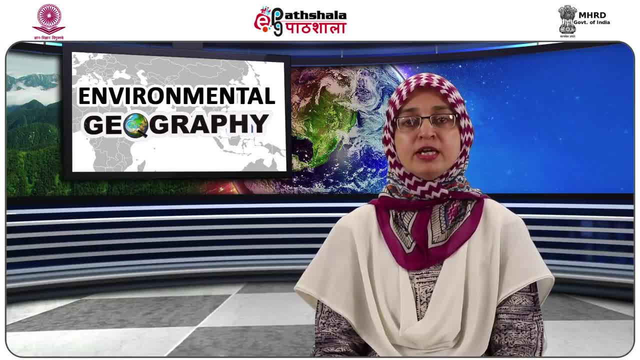 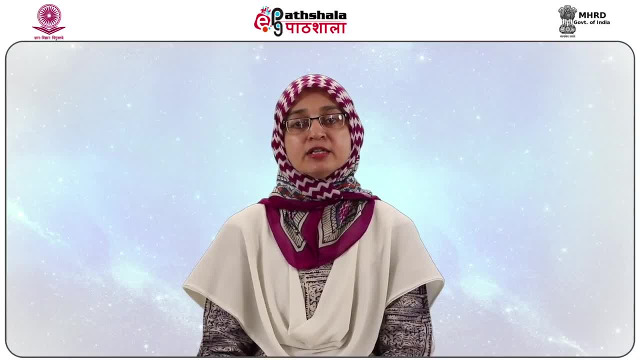 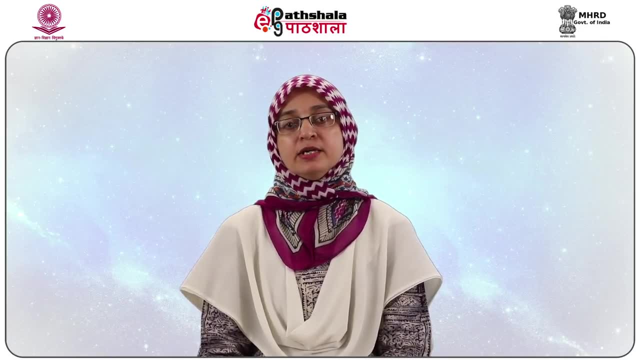 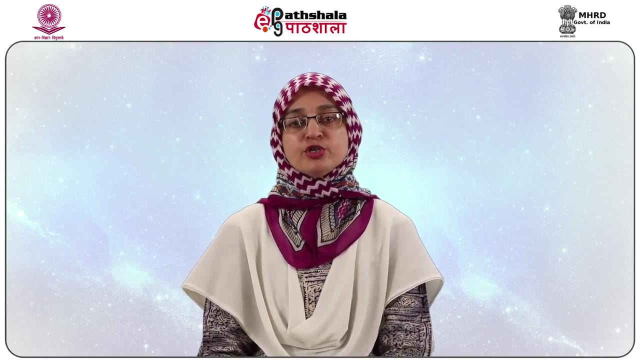 of the planet system In belief. at the very largest scale we can be determinist, whereas at the more local scales we can see the virtue of possibilism, or cultural and social determinism, And his teleological approach. Teachings of Judeo-Christian religious tradition promulgated the superiority of man to nature. 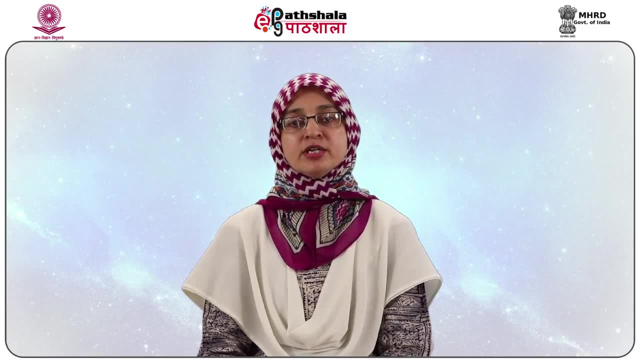 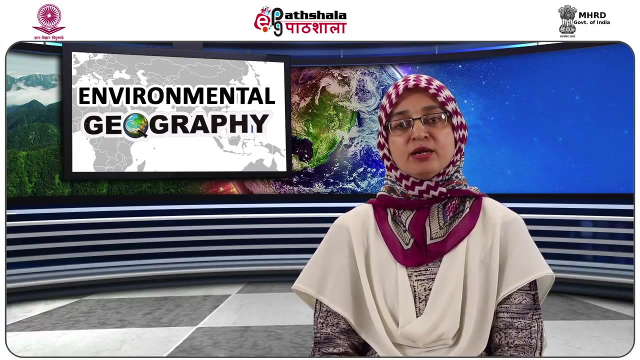 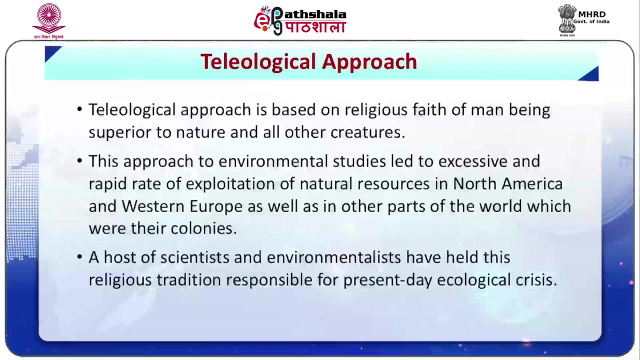 and all other creation, and that everything is created for his or her use and enjoyment. This idea fostered an inconsiderate exploitation by man of his natural environment. Environment today holds this religious tradition responsible for the environmental crisis. Teleological approach is based on religious faith of man being superior to nature and 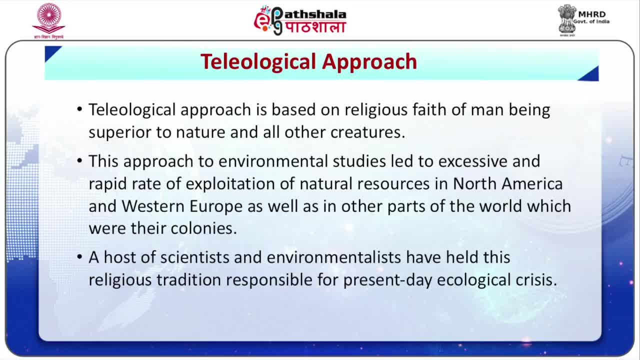 all other creatures. This approach to environmental studies, that is, man-environmental relationship, led to excessive and rapid rate of exploitation of natural resources in North America and Western Europe, as well as in other parts of the world which were their colonies. A host of scientists and environmentalists have held this religious tradition responsible. 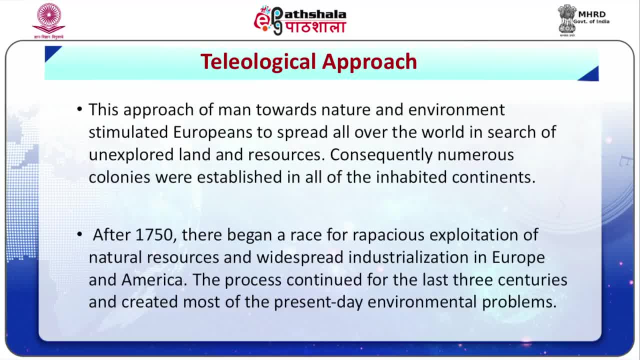 for present day ecological crisis. This approach of man towards nature and environment stimulated Europeans to spread all over the world in search of unexpected land and resources. END 0- KTIX. Consequently, numerous colonies were established in all of the inhabited continents After 1750, there began a race for rapacious exploitation of natural resources and widespread 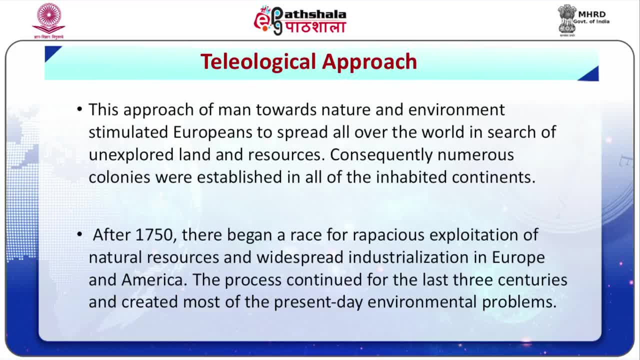 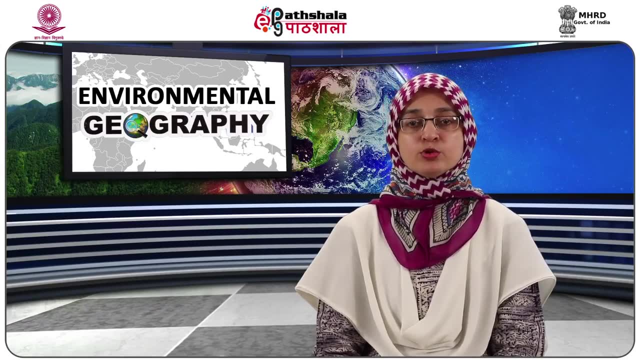 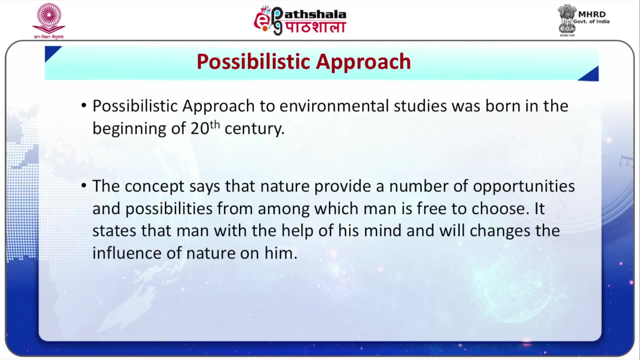 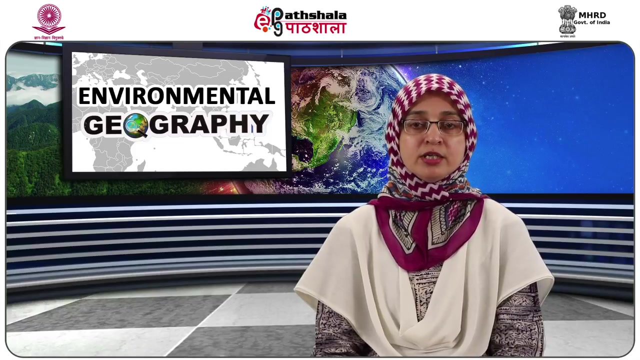 industrialization in Europe and America. The process continued for the last three centuries and created most of the present day environmental problems. Third is possibilistic approach. Possibilistic approach to environmental studies was born in the beginning of 20th century. The concept of determinism, which was conservative, cannot be accepted by a society which is civilized. 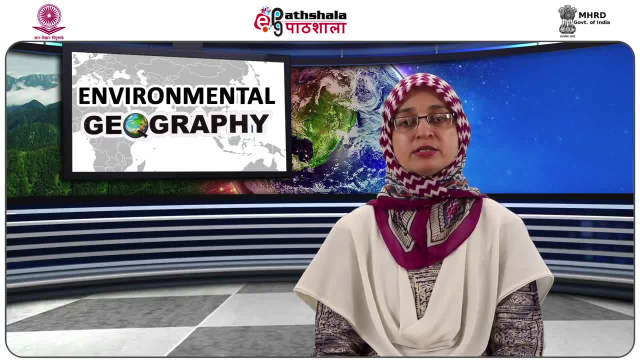 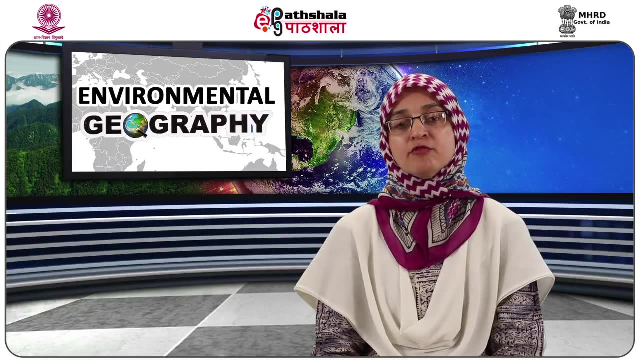 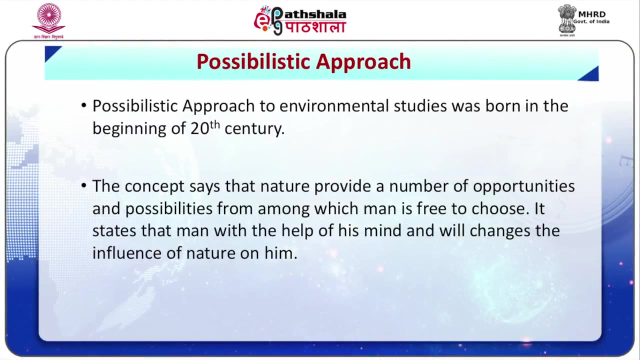 and advanced. The reason behind this is that man, with the help of technological development, has modified the nature of the environment. For example, he has created canals for making the water available in the extreme desert areas, for making it suitable for living. The concept of possibilism says that nature provide a number of opportunities and possibilities. 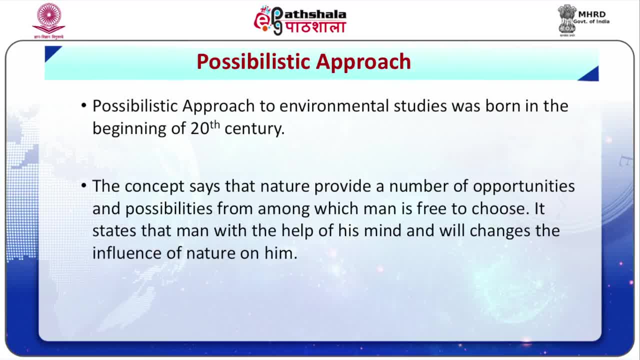 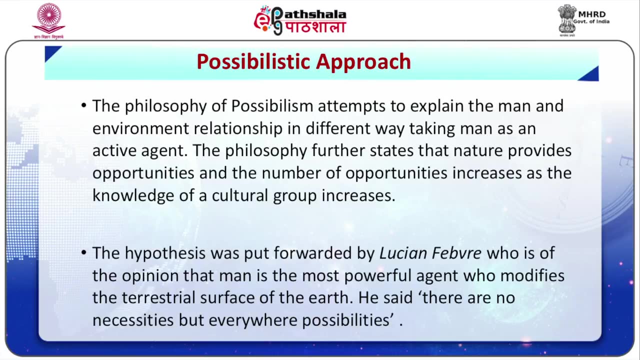 from among which man is free to select or choose. The philosophy states that man, with the help of his mind and will, changes the information influence of nature on him. The philosophy of possibilism attempts to explain the man and environment relationship in different way, taking man as an active agent. 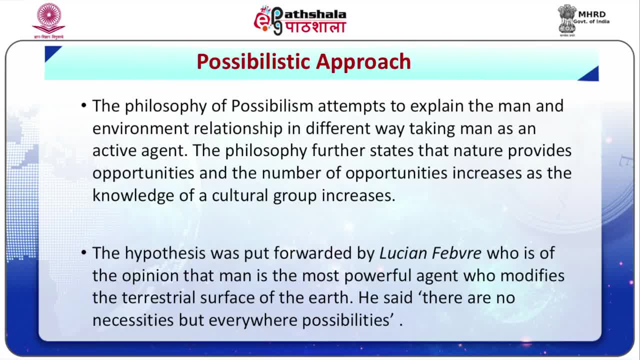 The philosophy further states that nature provides opportunities, and the number of opportunities increases as the knowledge and technology of a cultural group increases. Next slide, Next slide, Next slide: Possibilism was put forward by Lucian Favre, who is of the opinion that man is the most. 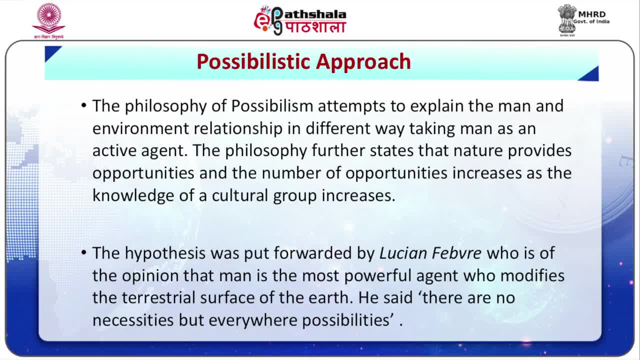 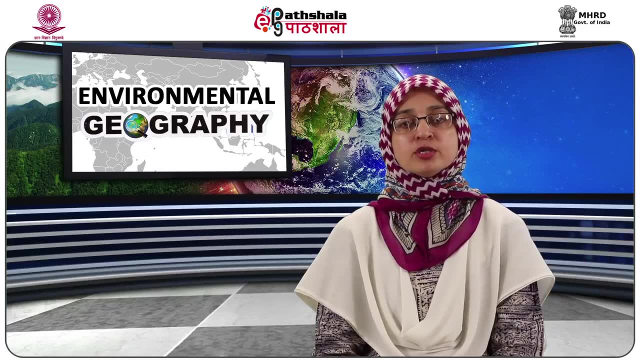 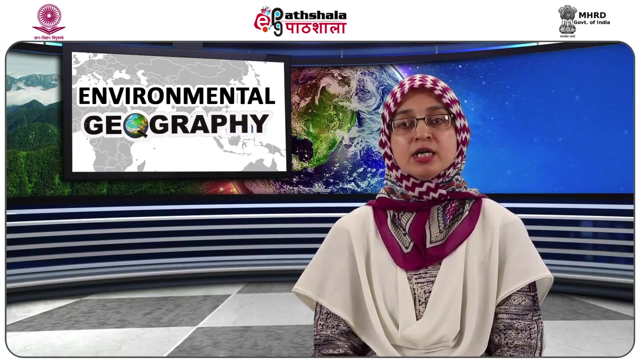 powerful agent who modifies the terrestrial surface of the earth. Lucian said that there are no necessities, but everywhere possibilities. For example, man invented iron and it was up to him that how he make the use of that iron. It was up to him whether he uses the iron for making hammer or a bicycle, a car, a ship. 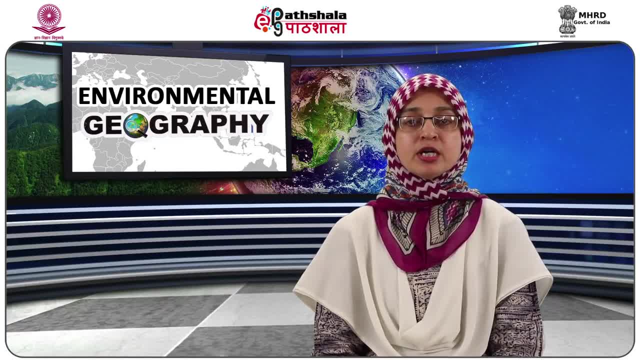 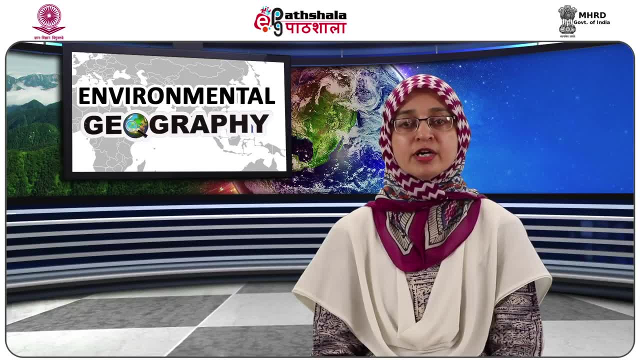 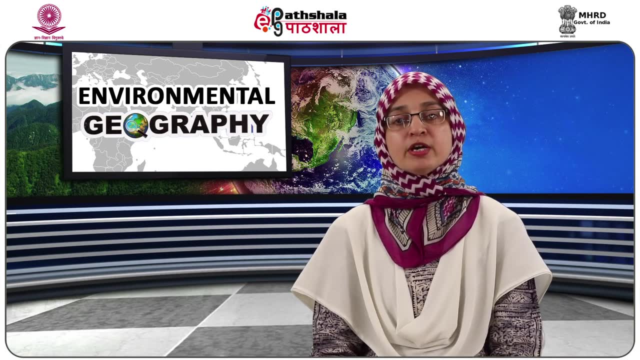 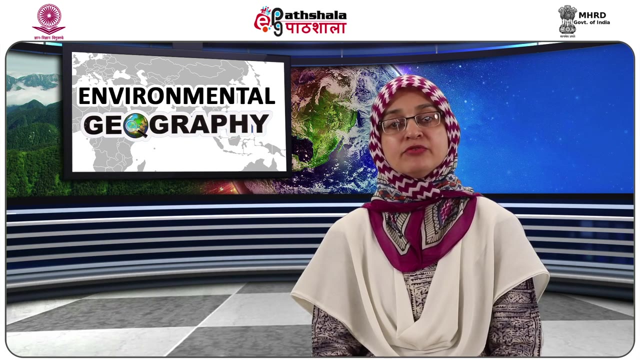 or a plane. it depends on his technological development. So the example proves that there are possibilities everywhere, but there are no necessities. Prior to the invention of iron, though, there was no necessity. There was no necessity for a plane, ship or a car, but possibilities were still there. 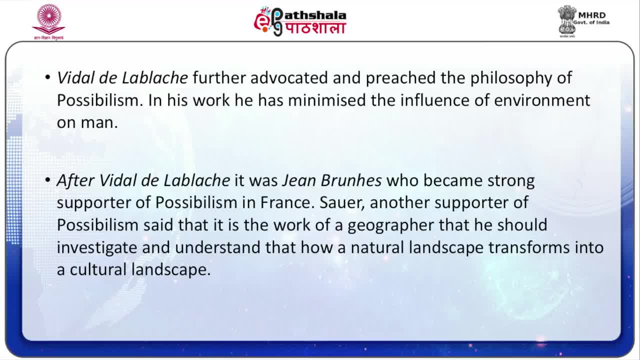 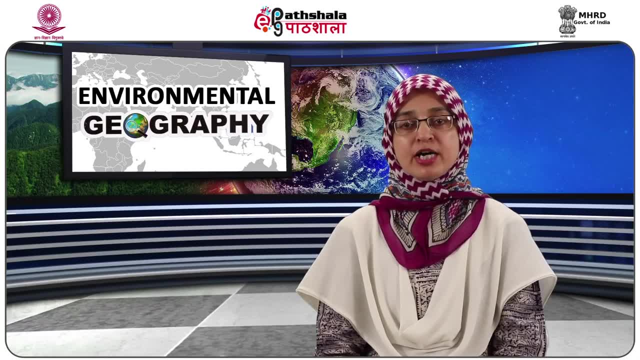 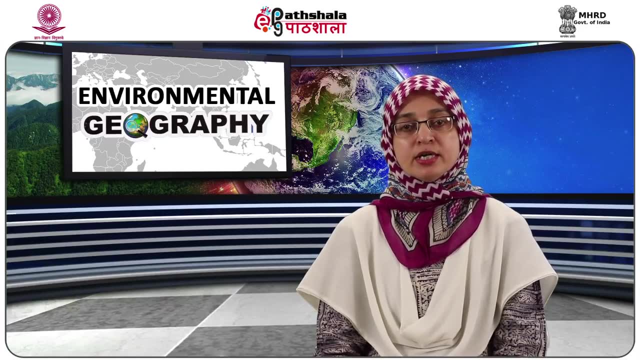 Weidel de la Blasch further advocated and preached the philosophy of possibilism. In his work he has minimized the influence of environment on man. He tries to explain the differences between groups living in the same environmental condition. He said that the differences are not because of the natural environmental conditions. 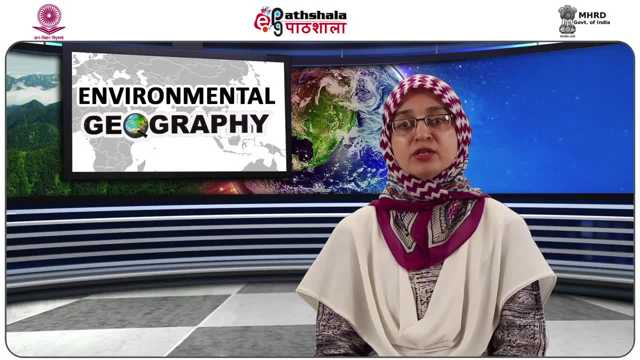 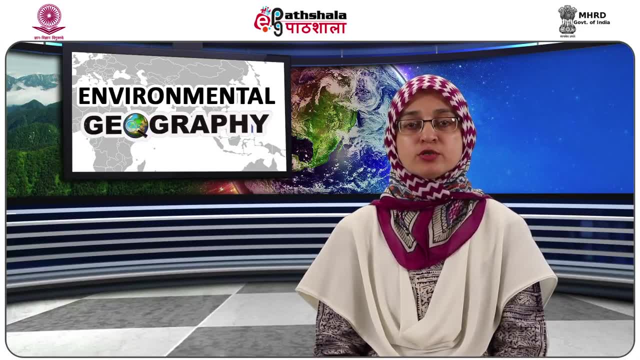 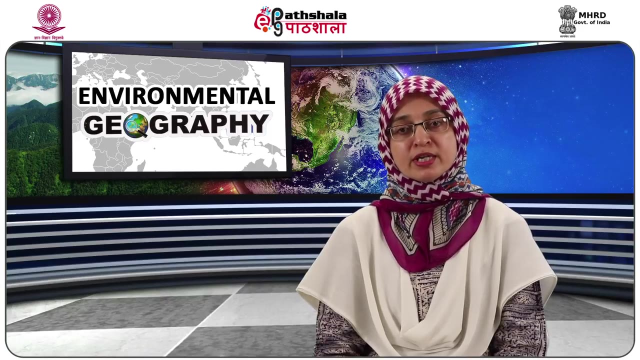 condition, but due to the variation in the attitude, values and habits of man. The possibilistic school of thought tries to explain the differences in human society on the basis of man himself bringing the changes and influencing the environment. and it is not only the nature solely responsible for bringing the changes or differences in. 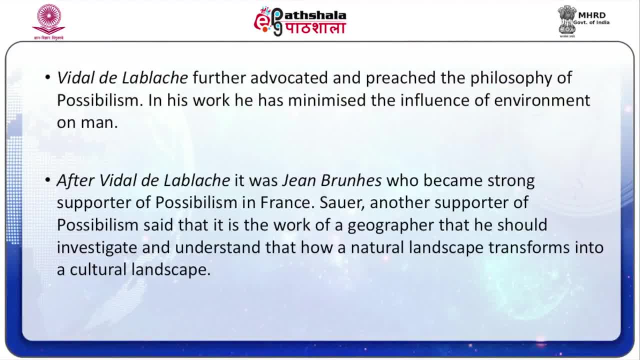 human society. After Vidal de la Blasch, it was Jean Bruns who became a strong supporter of possibilism in France. Saur, another supporter of possibilism, said that it is the work of a geographer that he should investigate and understand that how a natural landscape transforms into a cultural 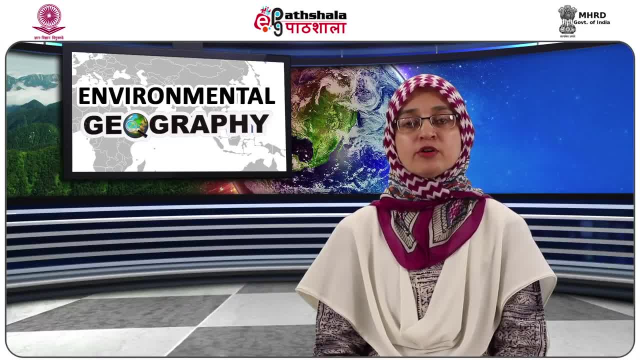 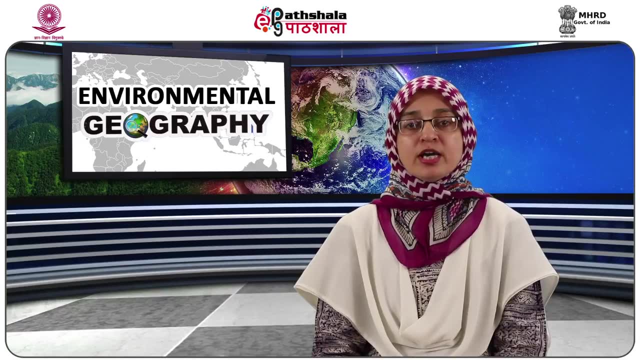 landscape. From such work, the geographer will be able to identify the major changes in the environment This particular area has resulted because of succession of human groups. For example, wheat does not have high yield where it was first domesticated, that is, South. 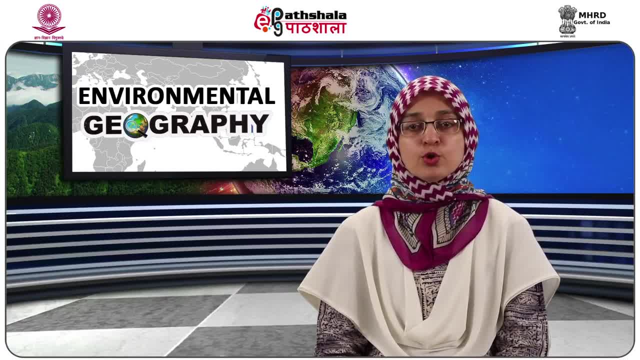 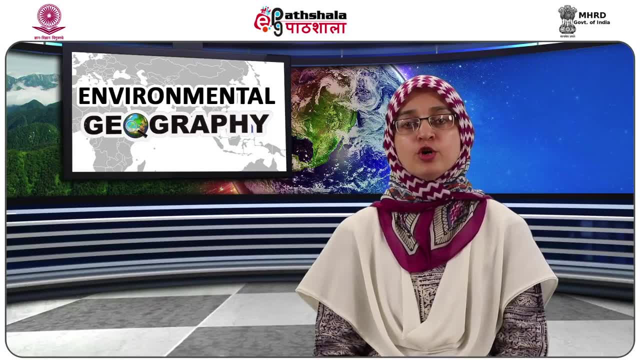 West Asia, but in America, Europe and some of the Asian countries. Thus, after the Second World War, the philosophy of environmentalism was attacked. Saur, another supporter of possibilism, said that it is the work of a geographer that he 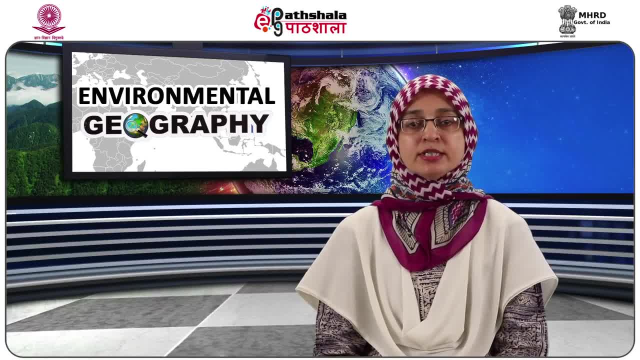 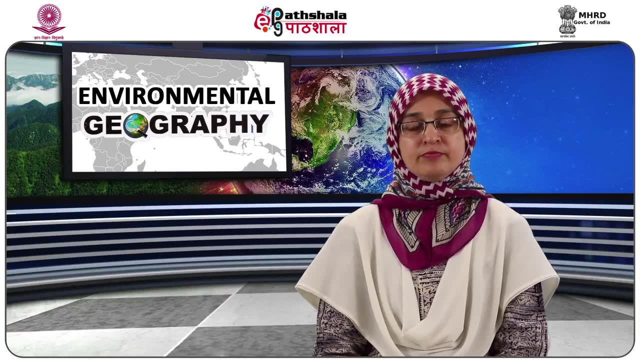 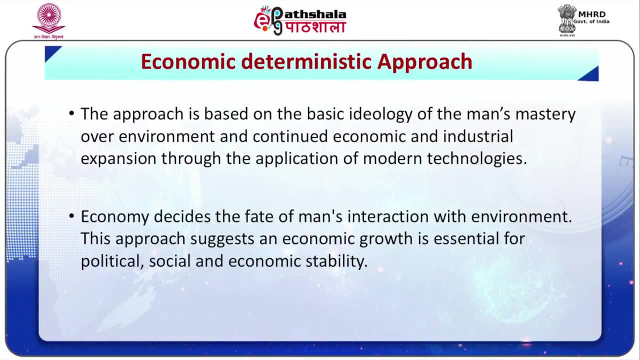 Many geographers in Britain, Canada and USA said that explanation of phenomena only on the basis of nature and its forces is incomplete and unsatisfactory until and unless man is included into it. Fourth is economic deterministic approach. This approach is based on the basic ideology of the man's mastery over environment and 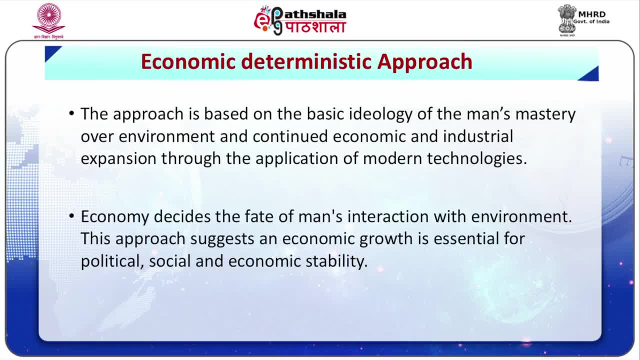 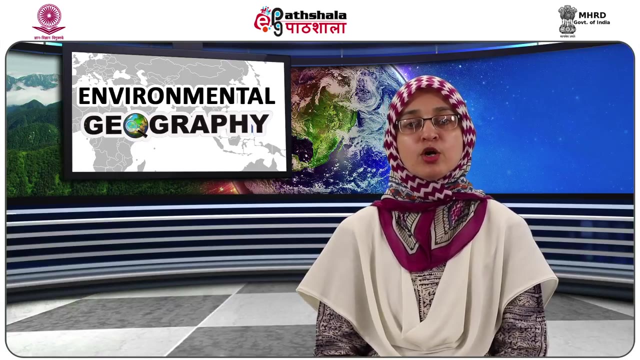 continued economic and industrial expansion through the application of modern technologies. Economy decides the fate of man's interaction with environment. This approach suggests an economic growth is essential for political, social and economic stability. The quality of environment normally assumes lower priority in planning. This approach based itself on two assumptions. firstly, positive correlation between the 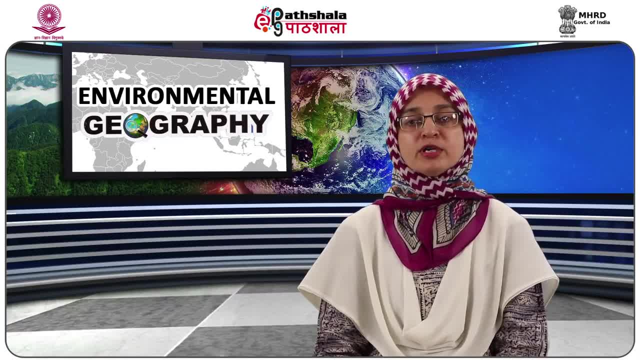 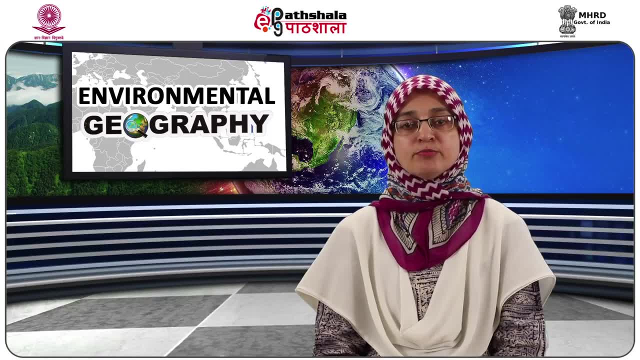 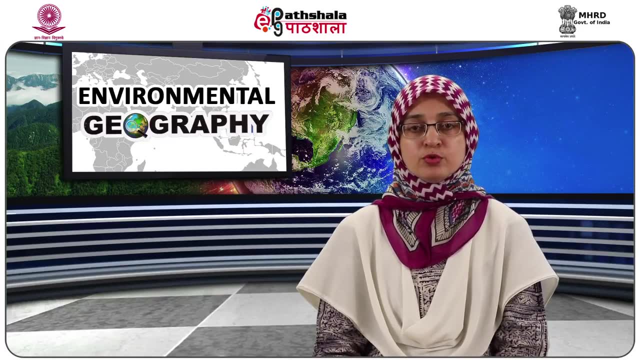 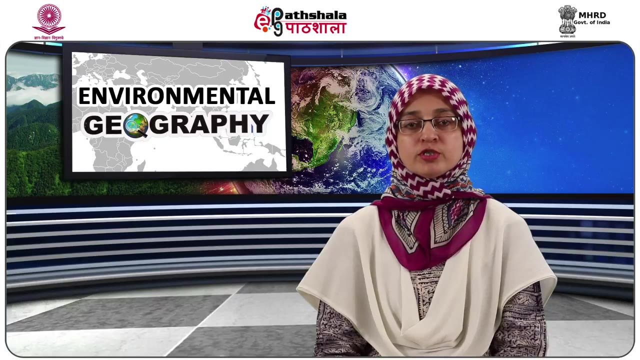 population of a green region and the level of economic development. Secondly, the interaction of people, resources and society are governed by universal economic principles. Now, fifth is regional approach. What is defined in regional approach? Regional approach is the region in contemporary terms, primarily as an object of study for 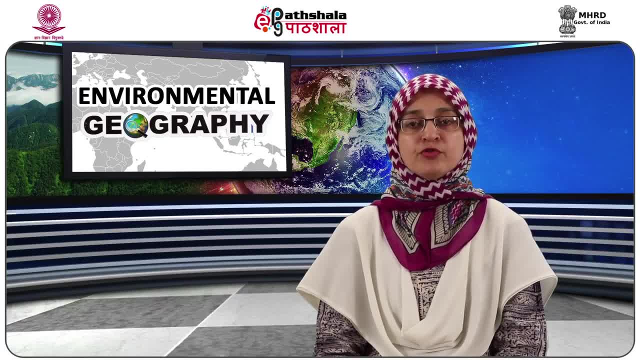 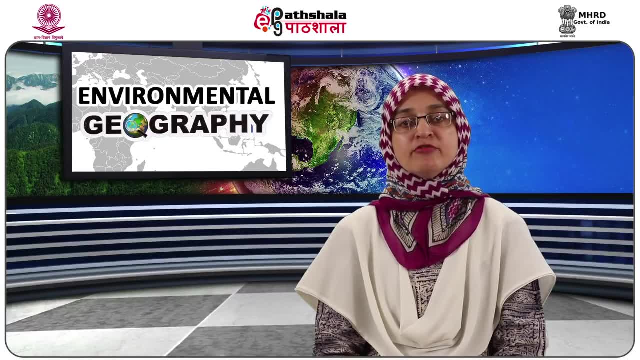 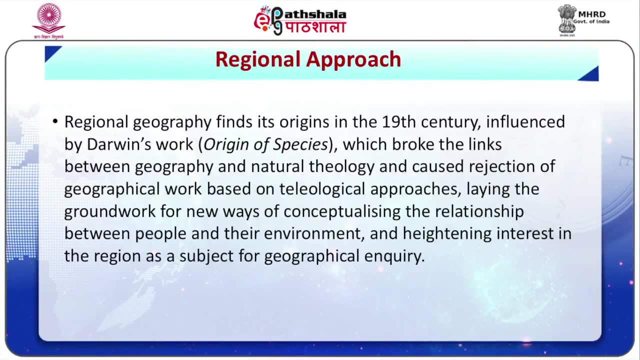 political and economic issues within human geography. In fact, the concept of region itself can be considered as having been born very much earlier within the discipline of geography. Regional geography finds its origin in the 19th century, influenced by Darwin's work, that is, Origin of Species, published in 1859. 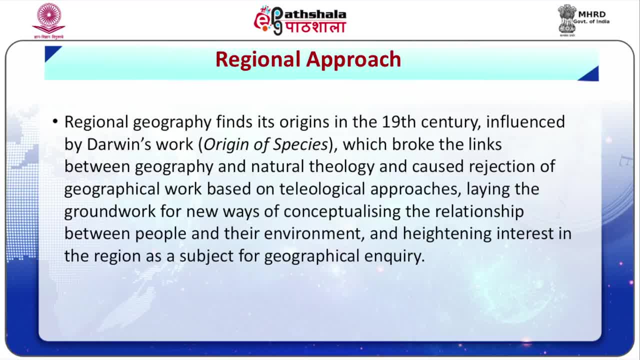 Regional geography finds its origin in the 19th century, influenced by Darwin's work, that is, Origin of Species, published in 1859. Which broke the links between geography and natural theology and caused rejection of geographical work based on teleological, Yayoi and at last호. 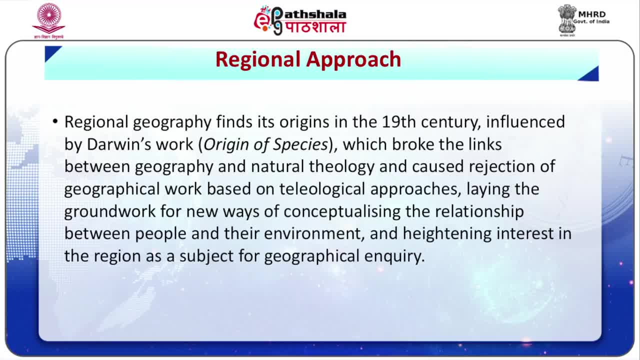 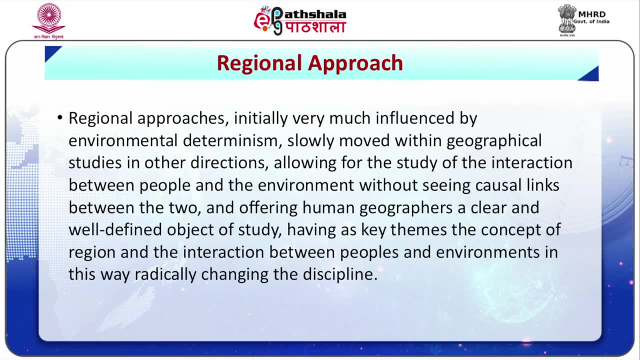 gyl approaches, laying the groundwork for new ways of conceptualizing the relationship between people and their environment and heightening interest in the region as a subject for geographical inquiry. Regional approach is initially very much influenced by environmental determinism. social issues slowly moved within geographical studies in other directions, allowing for the study of 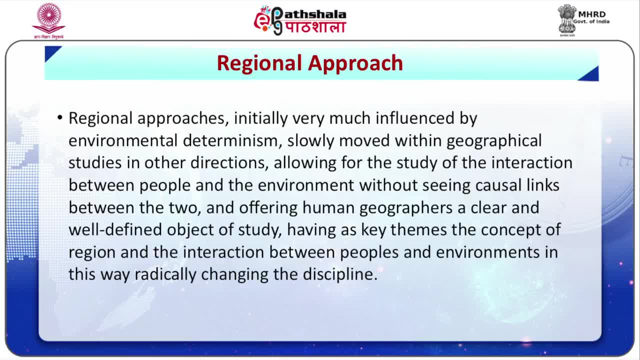 the interaction between people and the environment, without seeing causal links between the two and offering human geographers a clear and well-defined object of study, having as key themes the concept of region and the interaction between peoples and environments, in this way radically changing the discipline. 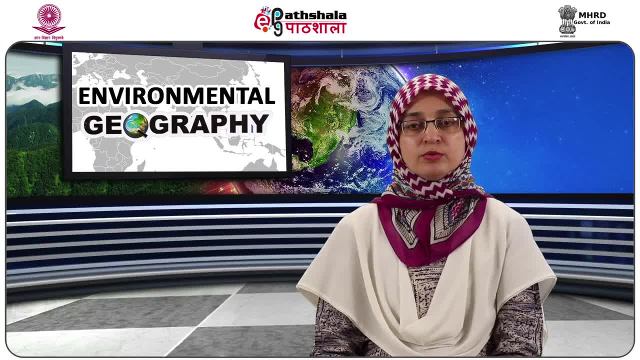 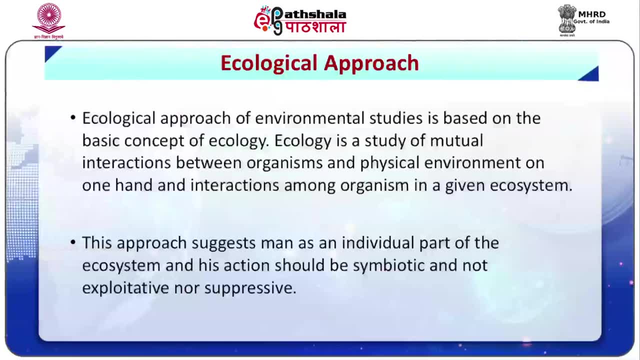 Six is ecological approach. Ecological approach of environmental studies is based on the basic concept of ecology. Ecology is a study of mutual interactions between organisms and physical environment on one hand, and interactions among organism in a given ecosystem. 6. Ecological approach. 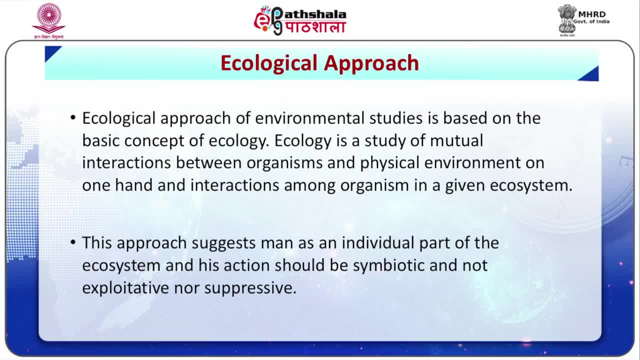 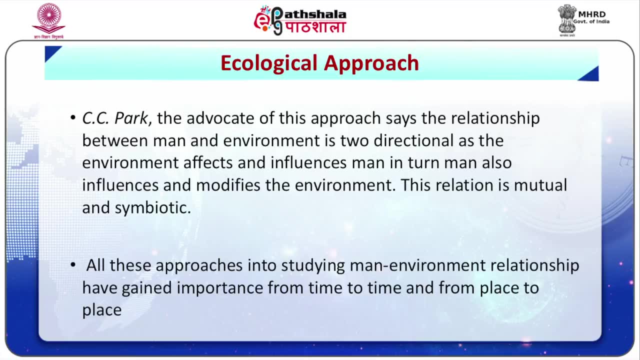 This approach suggests man as an individual part of the ecosystem and his action should be symbiotic and not exploitative nor suppressive. CC Park, the advocate of this approach, says the relationship between man and environment is two directional. as the environment affects and influences man, in turn, man also influences. 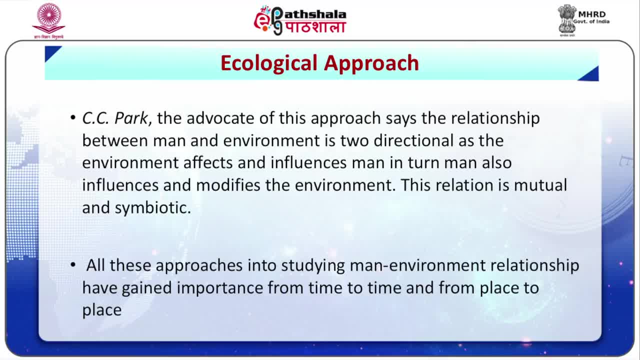 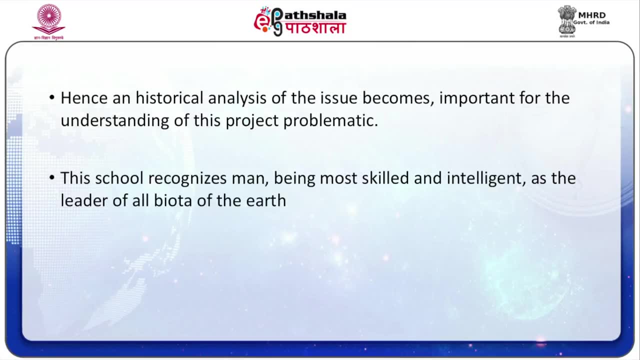 and modifies the environment. This relation is mutual and symbiotic. All these approaches into studying man-environment relationship have gained importance from time to time and from place to place. Hence an historical analysis of the issue becomes important for the understanding of this project problematic. 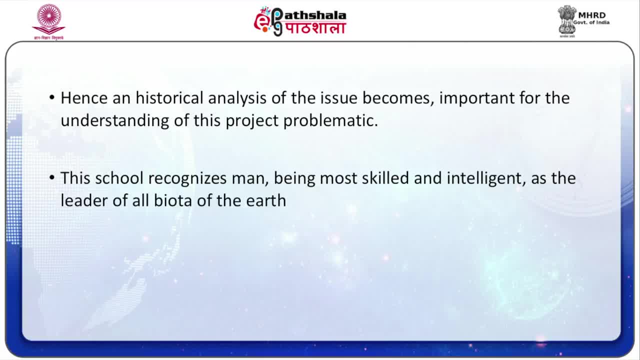 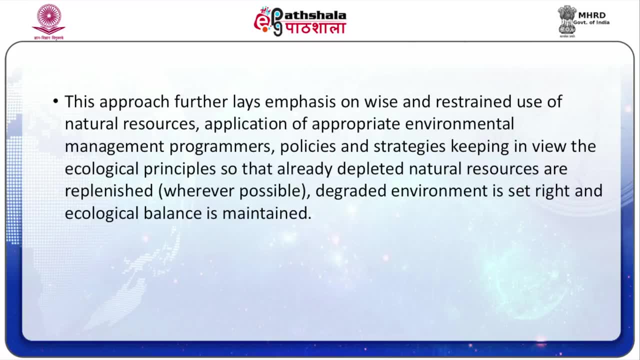 This school recognizes man being most skilled and intelligent. 7. Project problematic: This school recognizes man being most skilled and intelligent As the leader of all biota of the earth. This approach further lays emphasis on wise and restrained use of natural resources application. 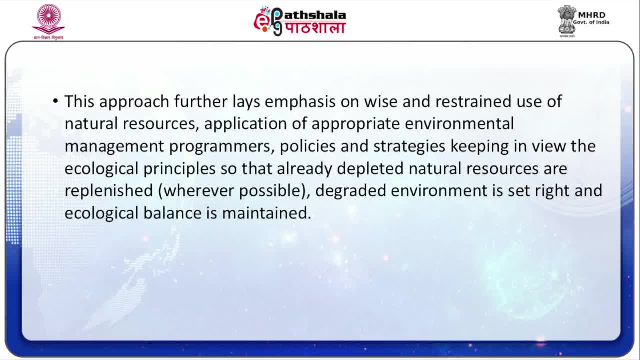 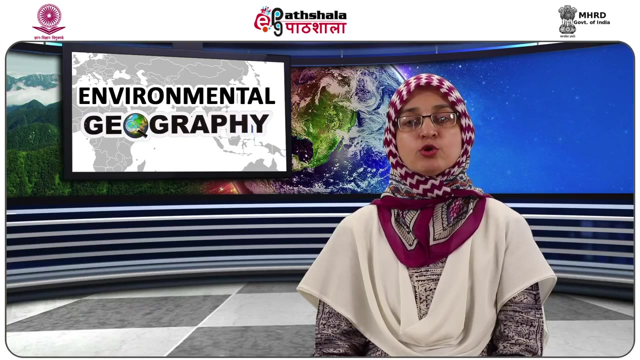 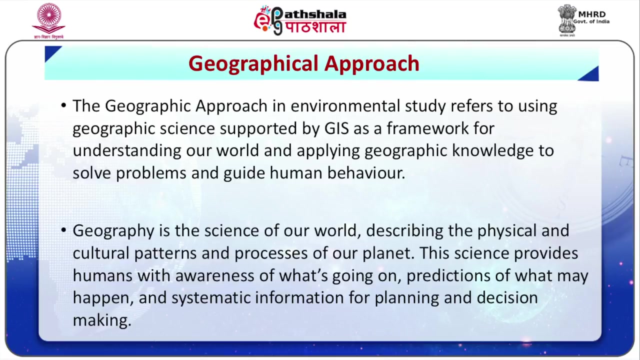 of appropriate environmental management programmers, policies and strategies, keeping in view the ecological principles, so that already depleted natural resources are replenished wherever possible, degraded environment is set right and ecological balance is maintained. Seventh is geographical approach. The geographical approach in environmental study refers to using geographic science, supported by GIS, as a framework for understanding our environment. 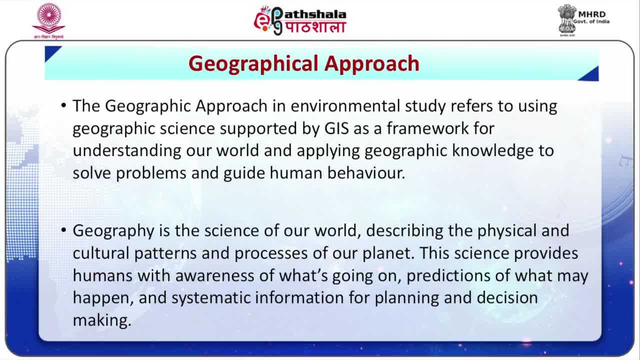 and applying geographic knowledge to solve problems and guide human behavior. Geography is the science of our world, describing the physical and cultural patterns and processes of our planet. This science provides humans with awareness of what's going on, predictions of what may happen and systematic information for planning and decision making. 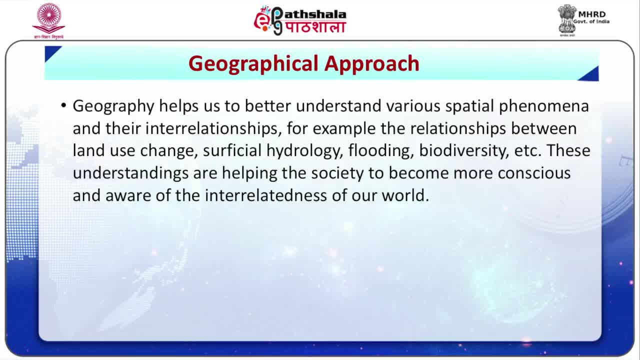 Geography helps us to better understand various spatial phenomena and their implications, For example, the relationships between land use change, surficial hydrology, flooding, biodiversity, etc. These understandings are helping the society to become more conscious and aware of the interrelationships of our world.